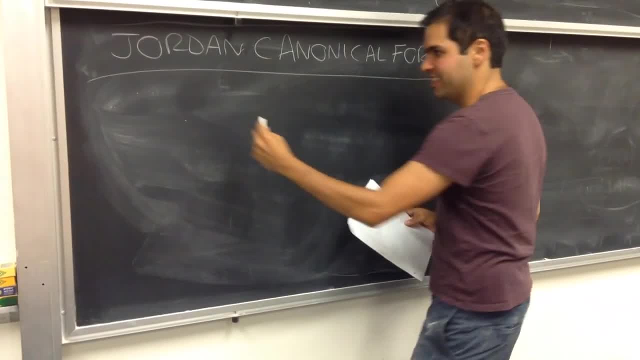 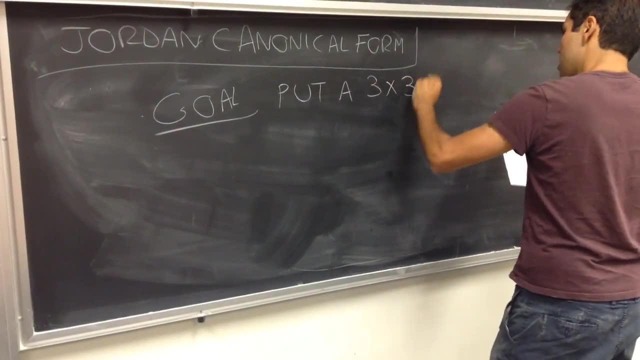 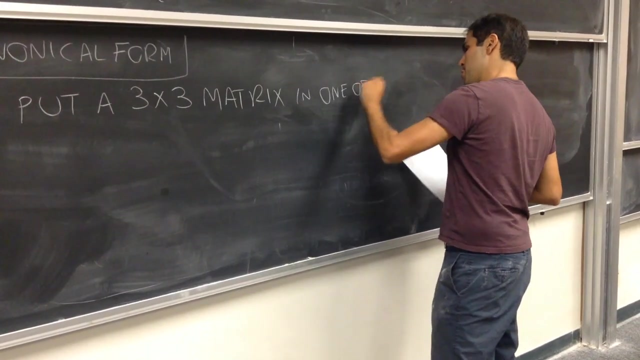 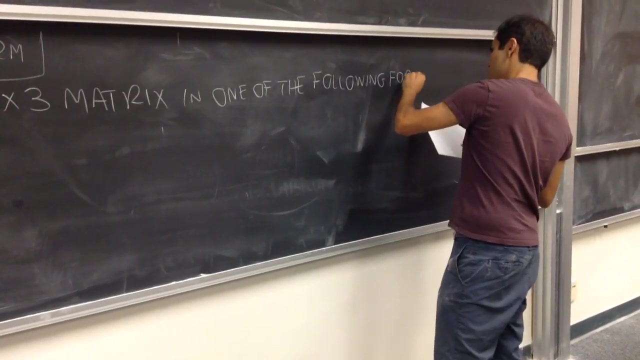 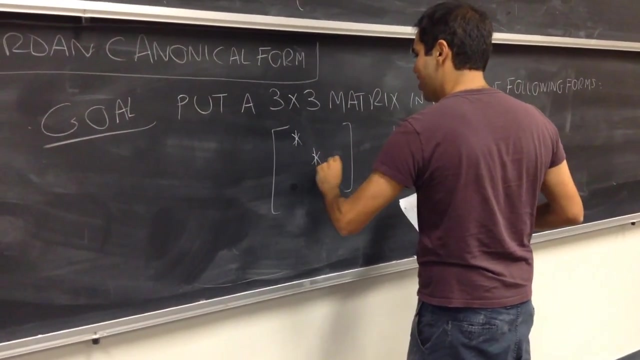 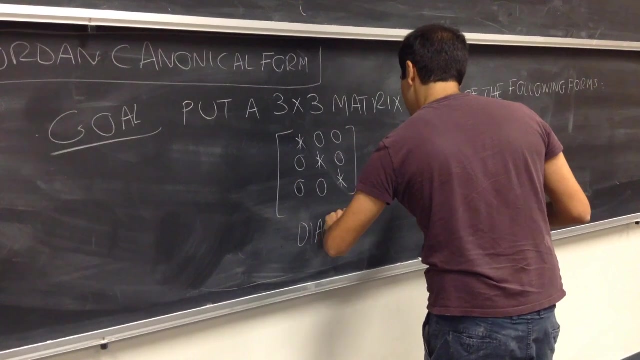 goal, And here we will focus on three by three matrices. Put a three by three matrix In one of the following forms: either a diagonal matrix, like something that looks like star, star, star and everything else is zero. that's diagonal, which is really the best possible. 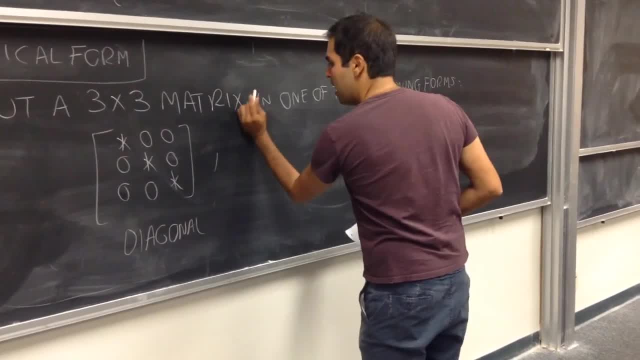 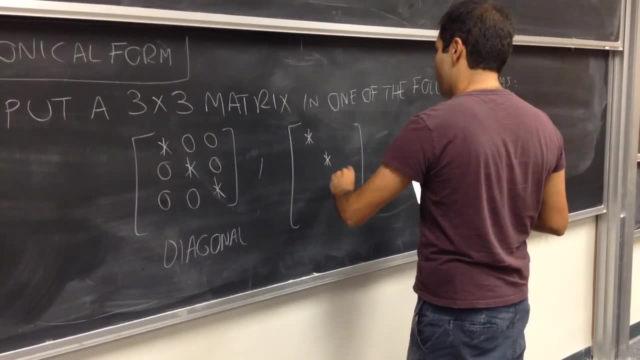 case, And I want you to think about this, And I want you to think about this, And I want you to think about this, and I'll talk about that. But it turns out sometimes you cannot put a matrix in this form, but you can still put it, in most cases, in some other forms. 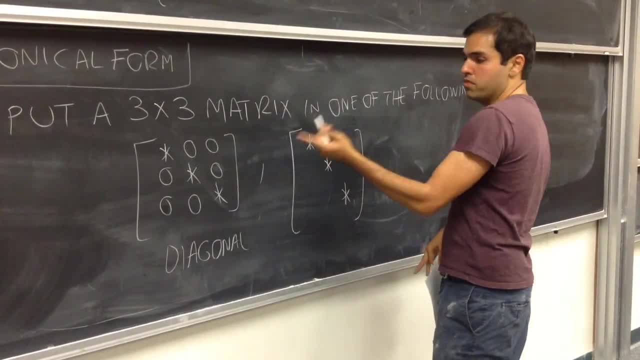 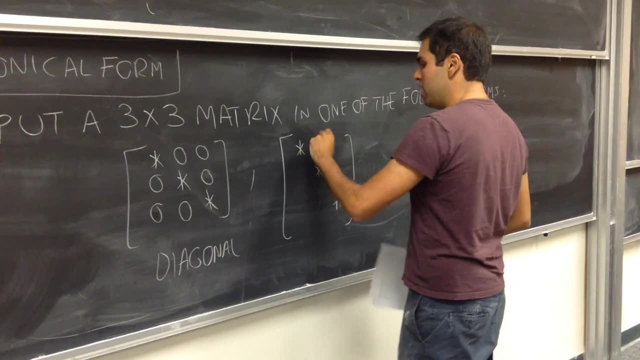 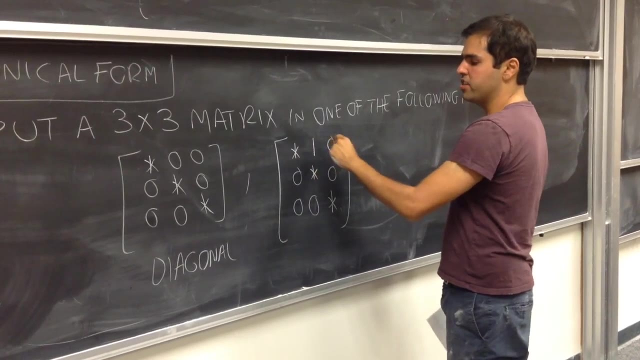 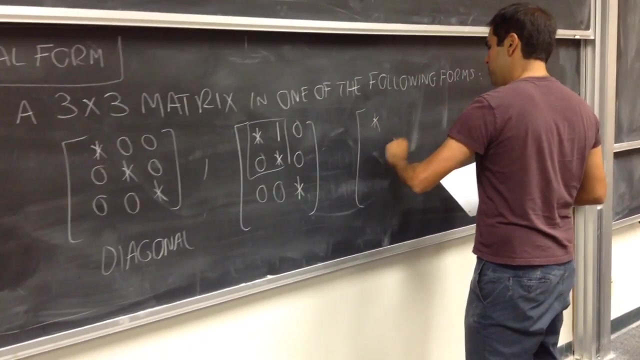 Maybe something where the diagonal terms can be whatever, but where all the other terms, well, they're not always zero, but most of them are, except maybe for a couple of ones. So in this thing we have a star, and you call this a Jordan block. And let me tell you another scenario: maybe star, star, star. 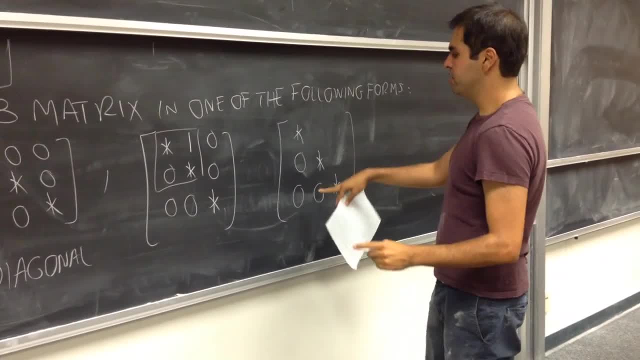 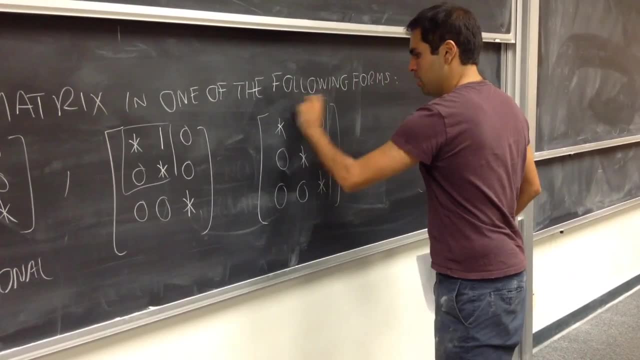 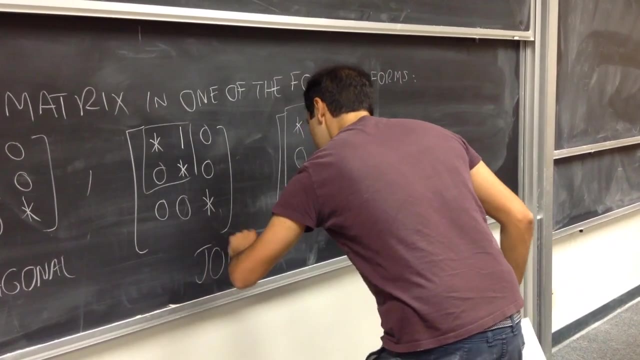 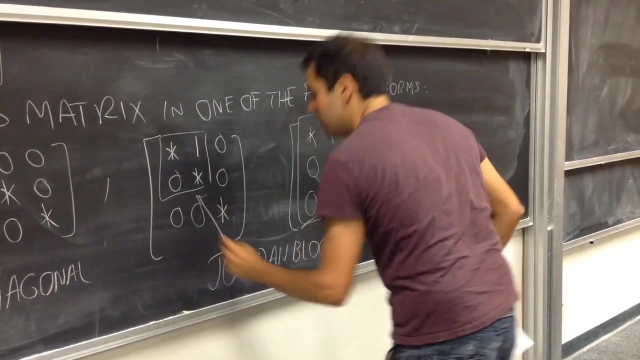 where everything below the diagonal is zero, but just all the entries exactly above the diagonal. they're one, And those cute blocks with stars and one. as I said, we'll call them Jordan blocks. Let me guide you through some examples of all the possible scenarios that could happen. 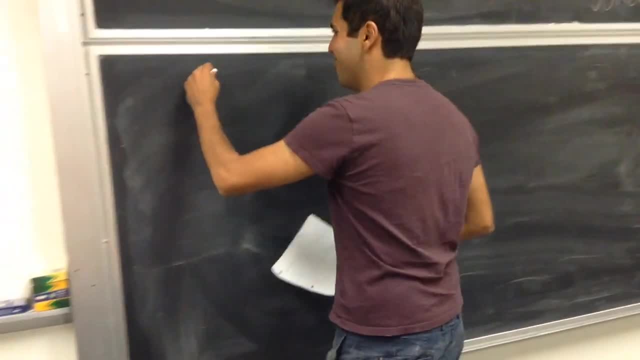 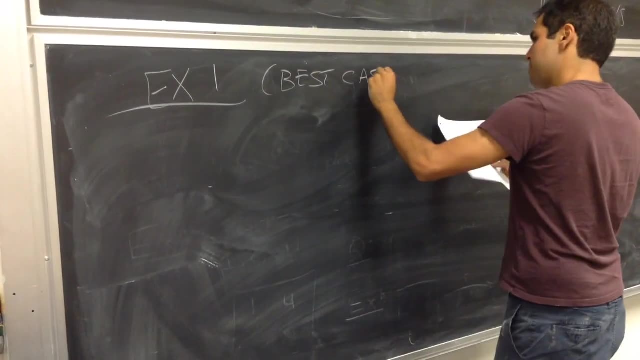 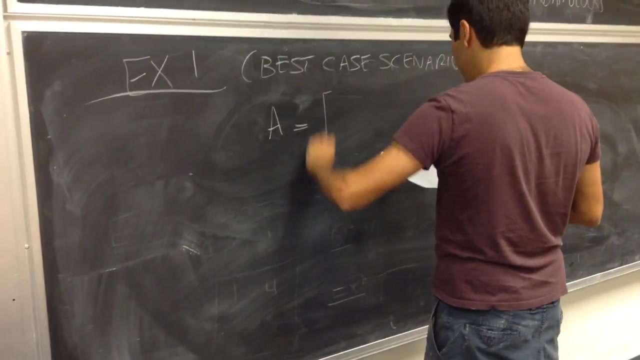 First example: best case scenario. unfortunately not always happens. scenario: Best case scenario: Suppose you have the matrix A, which is 4, 0, 1, 2, 3, 2, 1, 0, 4.. 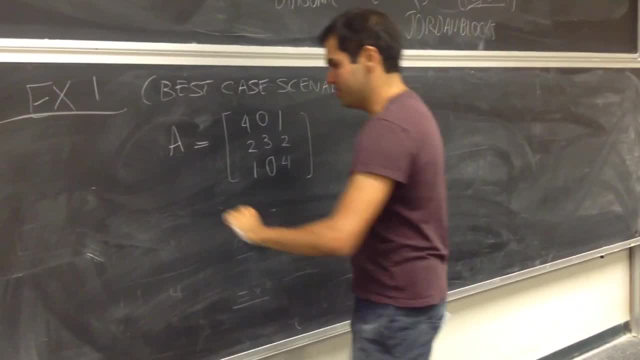 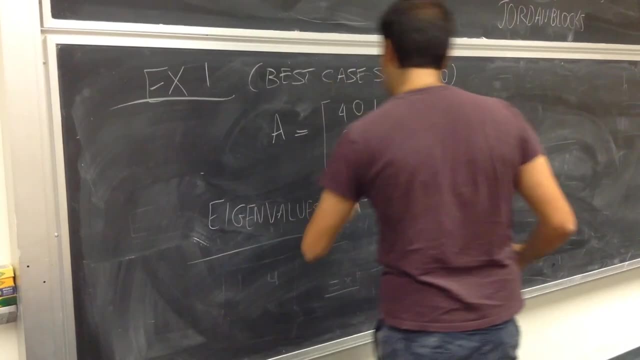 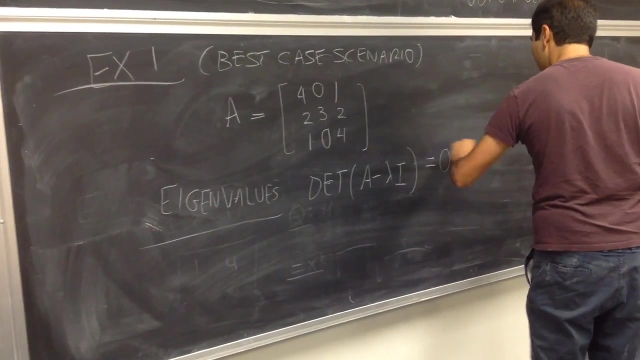 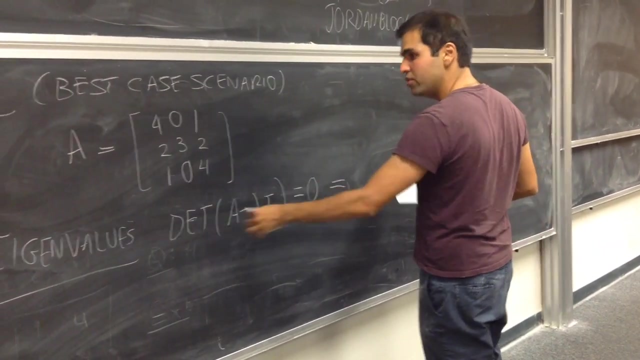 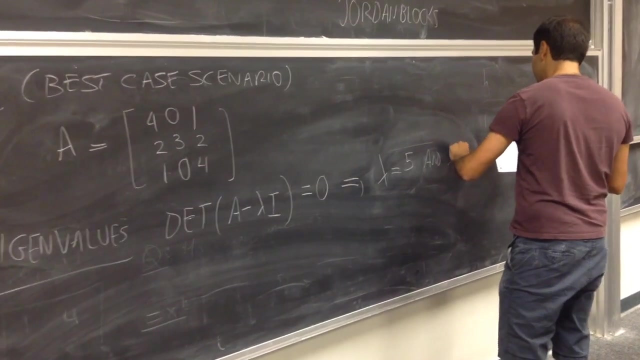 Suppose you find the eigenvalues. eigenvalues, which means you solve the determinant of A minus lambda, I equals to 0. Again, I will not do this computation because otherwise this video will be too long. but let's say you do this. you find that lambda equals to 5 and lambda equals to 3.. 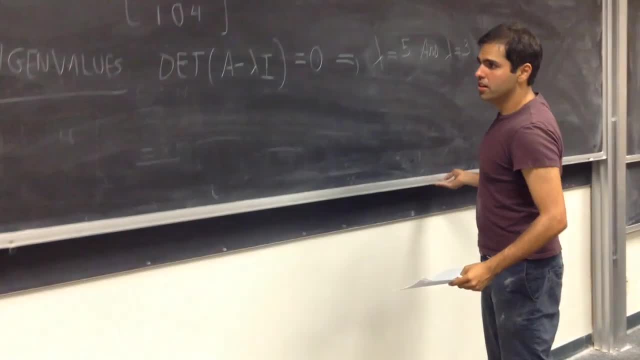 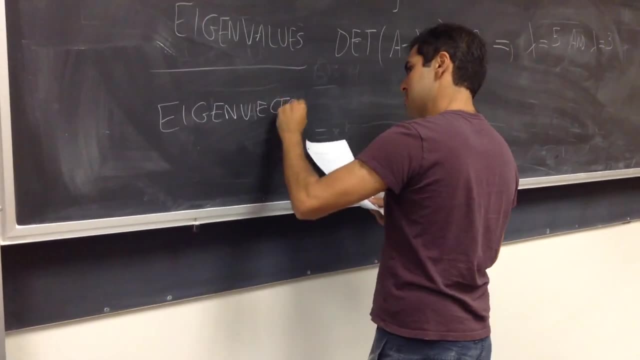 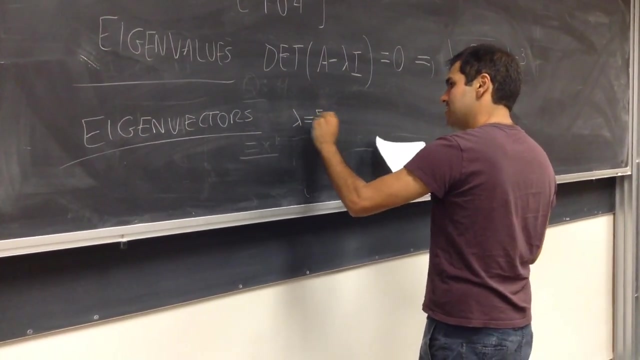 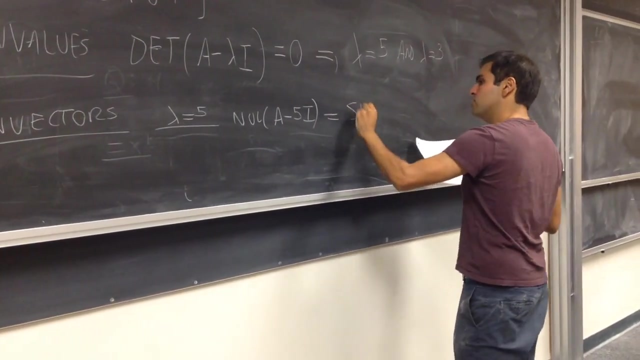 Once you find the eigenvalues, you find the eigenvectors. So for both of them you find, For both of them you find. For both eigenvalues, you find the corresponding null spaces. So lambda equals to 5.. If you find the null space of A minus 5I suppose you do this and you find that it's the span of. 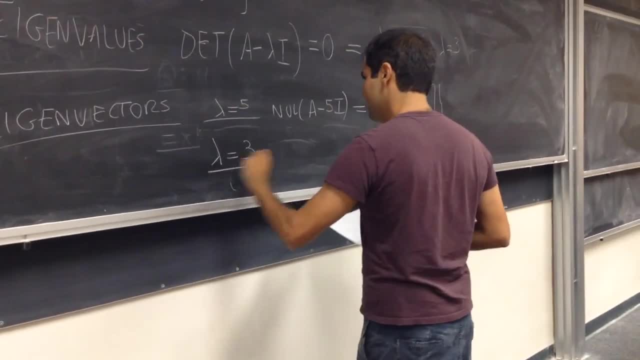 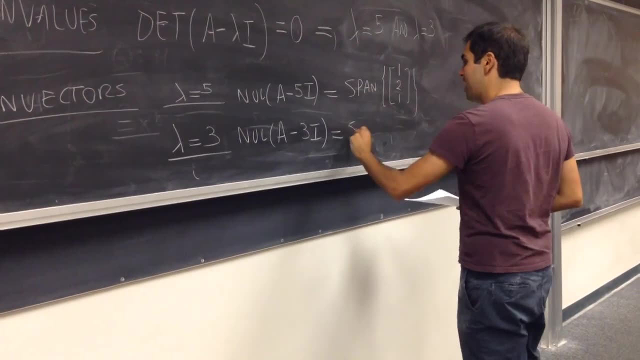 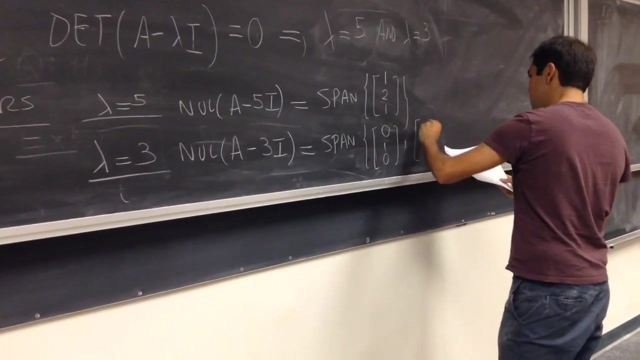 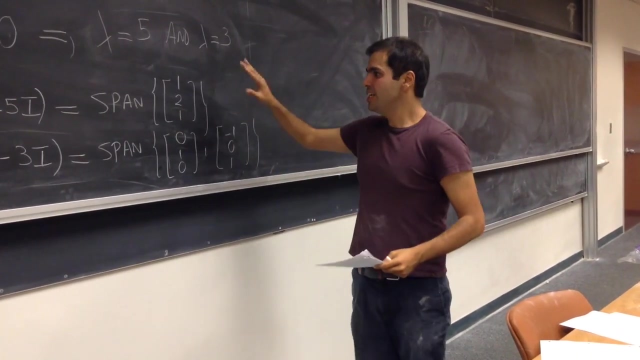 and then for lambda equals to 3, suppose you do the null space of A minus 3I and you find after some calculations that you get the span of of 0, 1, 0 and minus 1, 0. This is amazing because you found three eigenvectors. so 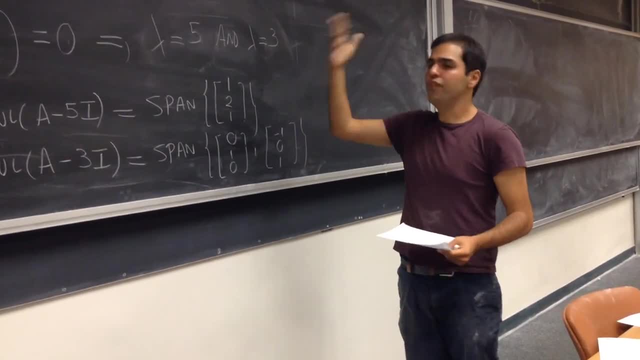 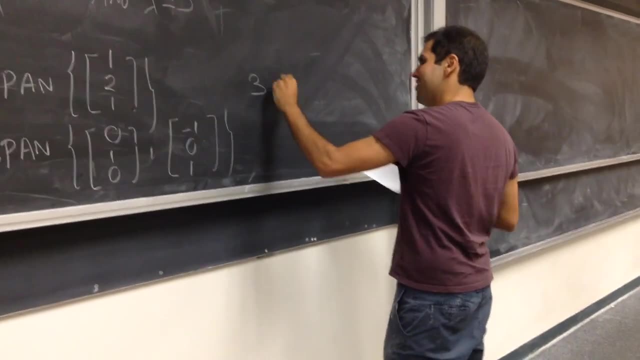 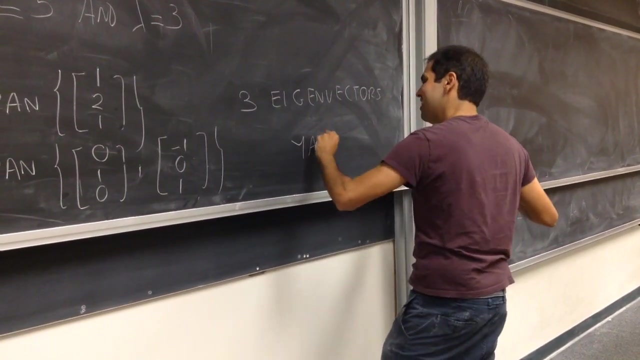 three linearly independent eigenvectors and you have a 3 by 3 matrix. So this is great. so three linearly independent eigenvectors- Yay. That's where, like fireworks should like come into your mind, because this is really the best possible. 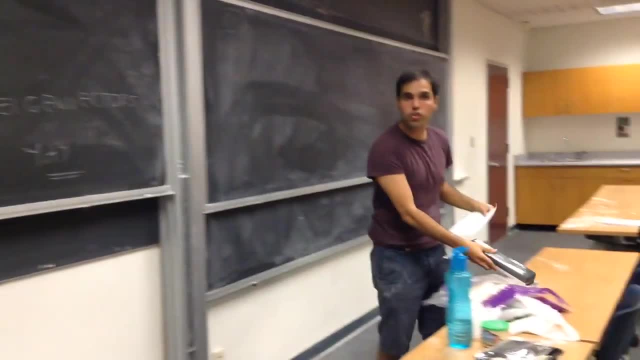 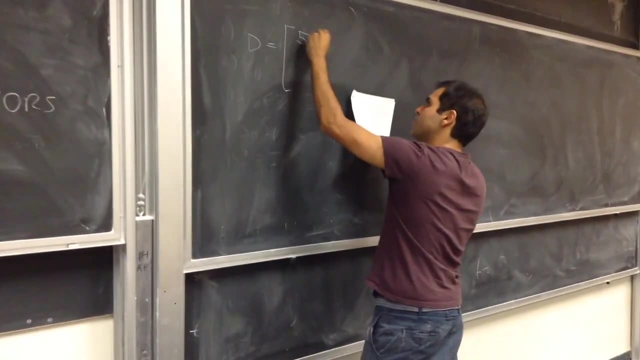 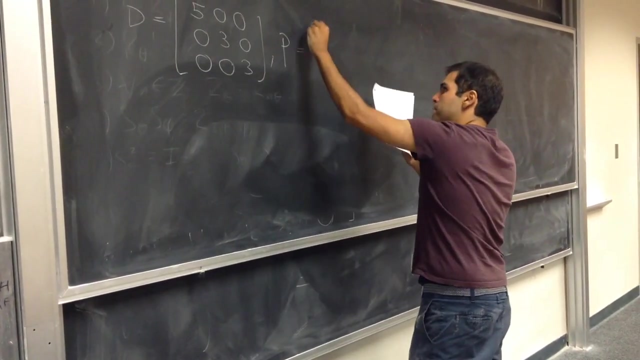 scenario. Why? Because you can just put your matrix in diagonal form. namely, if you find, if you have d equals to the matrix of eigenvalues. so 5 by 0,, 0,, 0,, 3,, 0,, 0,, 0, 3, and p be the matrix of corresponding eigenvectors. So for 5, you put: 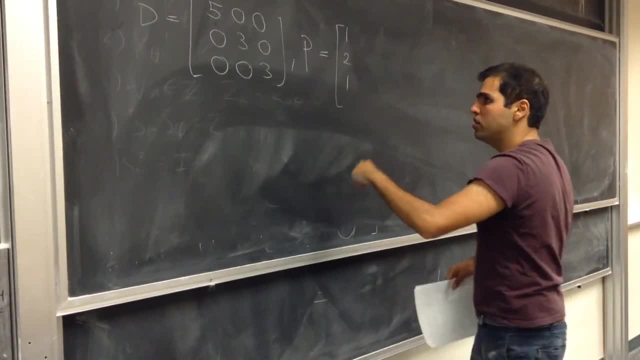 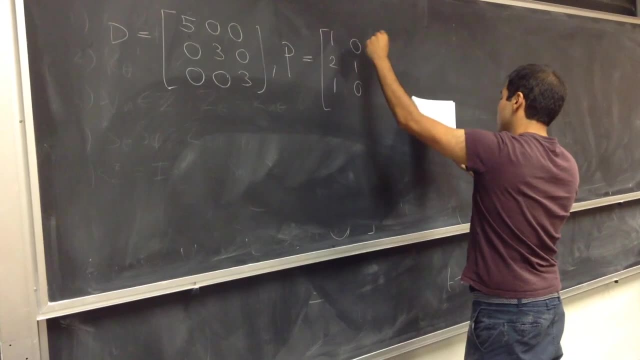 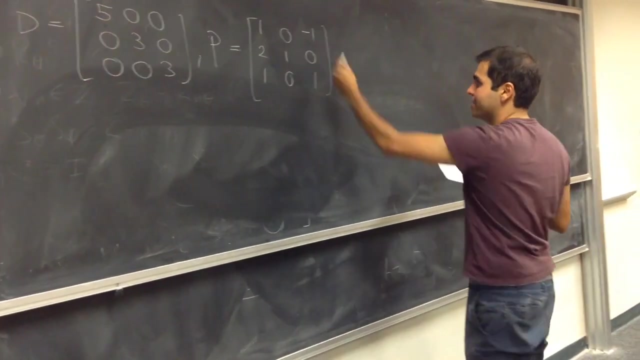 the eigenvector corresponding to 5,, so 1,, 2,, 1, and for 3, you put the two other eigenvectors, doesn't matter which order. okay, 1, 0,, 1, 0, minus 1, 0, 1, and then you get in fact. 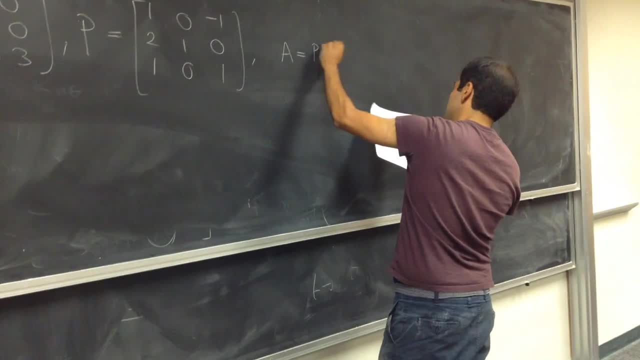 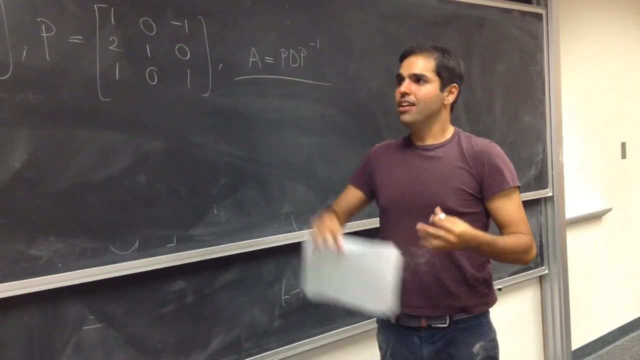 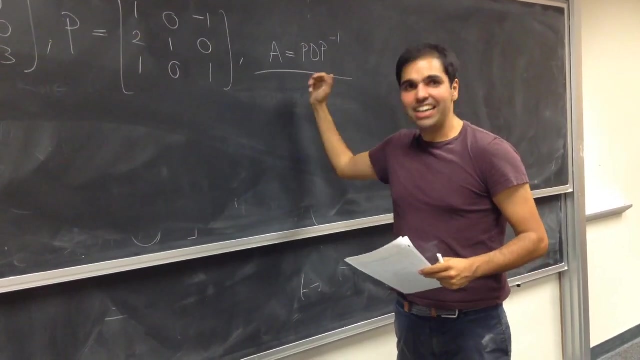 you know by a theorem that a equals to pdp. And this is the case where we say a is diagonalizable, namely we can put a into, we can transform a into a diagonal matrix. This is great but, as I said, it won't always happen. especially on your exams, it might not happen. 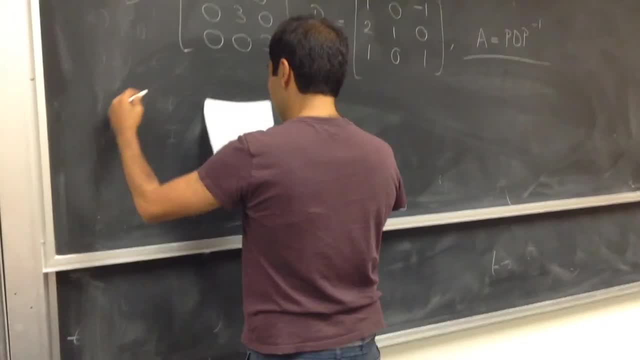 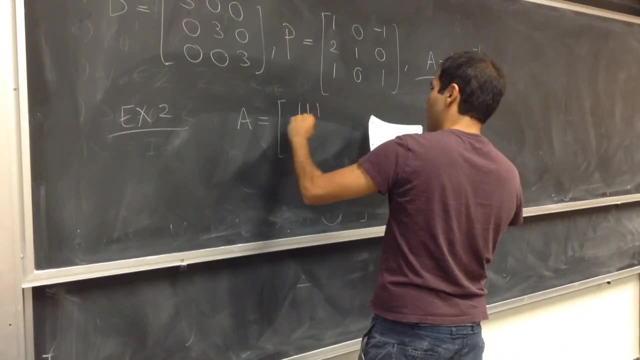 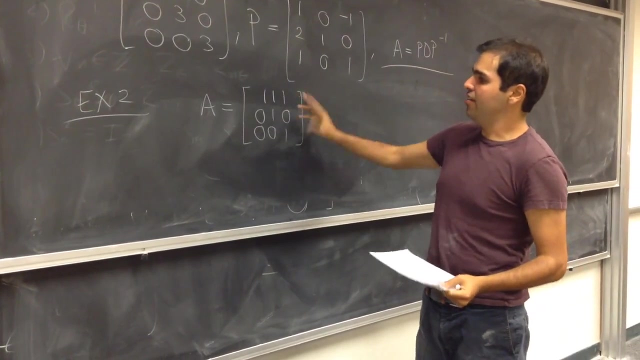 and let's see what happens, you know, in other cases. So what about the following example? A equals to 1, 1, 1, 0, 1, 0, 0, 0, 1.. Well, you might say, hey, it looks like a Jordan block. 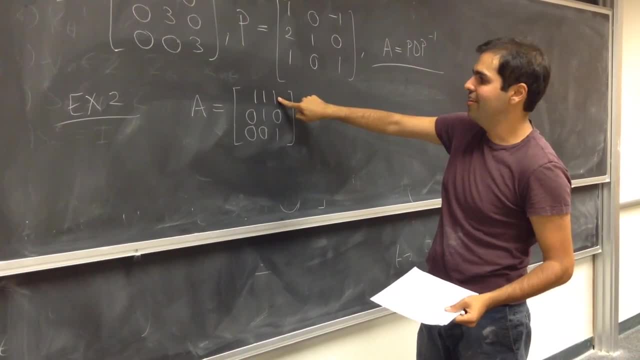 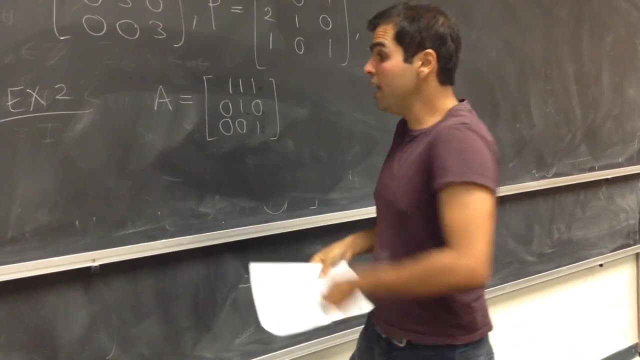 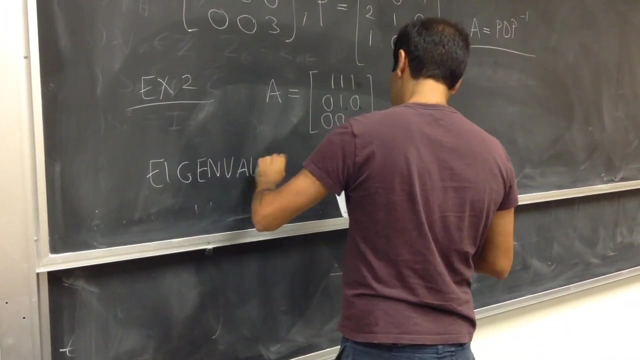 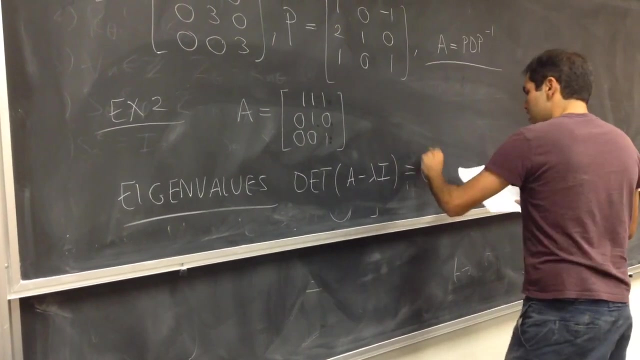 not quite, because for Jordan blocks this has to be 0. It's only values exactly above the diagonal. that could be 1s. Okay, well, let's see where the problem is. Let's find the eigenvalues Determinant of a minus lambda i. You do this not hard, because this is upper triangular. 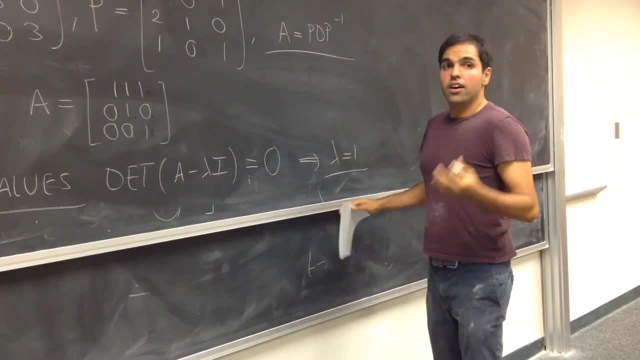 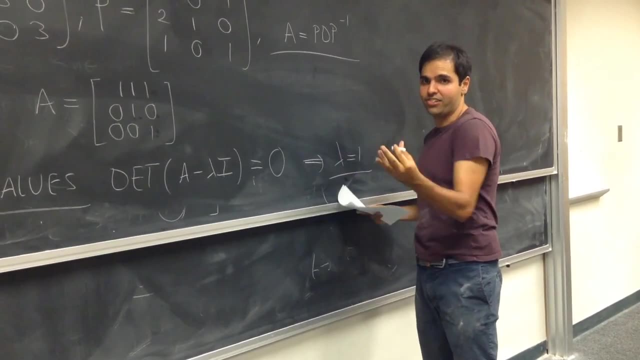 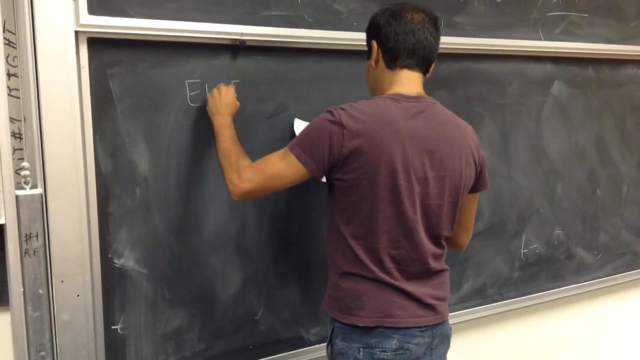 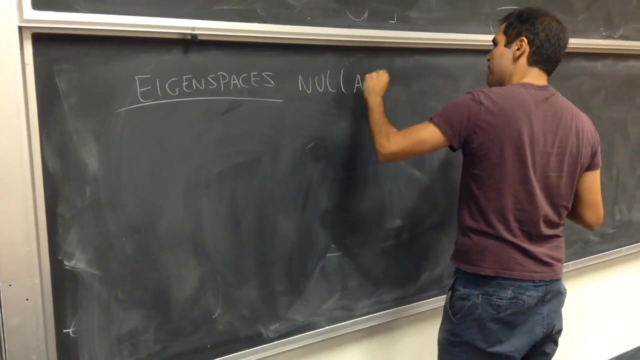 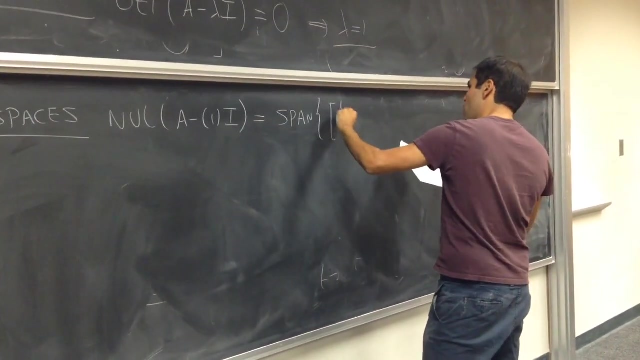 and you get that lambda equals to 1.. No need to despair, it could happen. it will not happen that you could still get three eigenvectors. But let's see, let's find the eigenspaces, So null space of a minus 1i, that's. if you do this, let's say you get the span of 1, 0, 0, 0, 1 minus 1.. 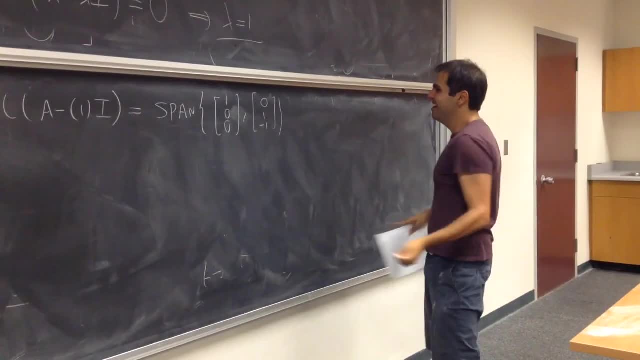 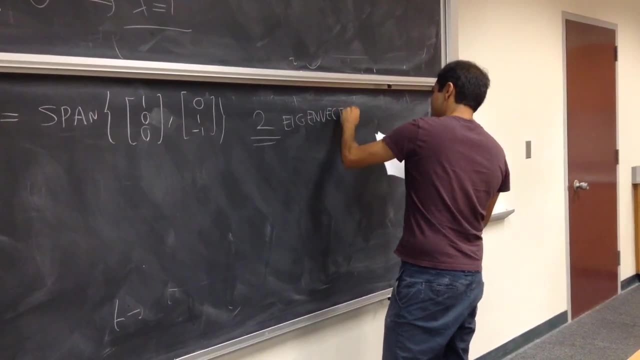 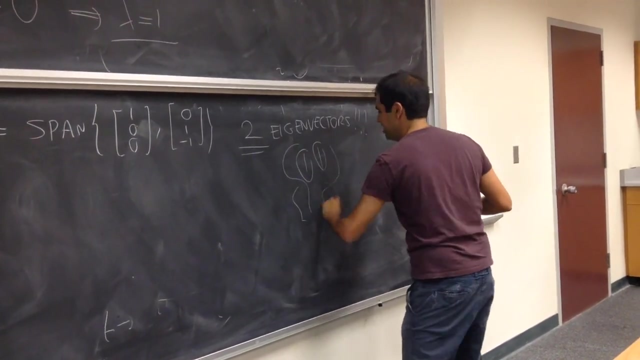 Oh no, How bad we only have two eigenvectors. Sure, it's not going to be too hard. Sure, Sure, Sure, Sure. So you have this chopped space like: ahhh, this scream thingy, you know this scream. 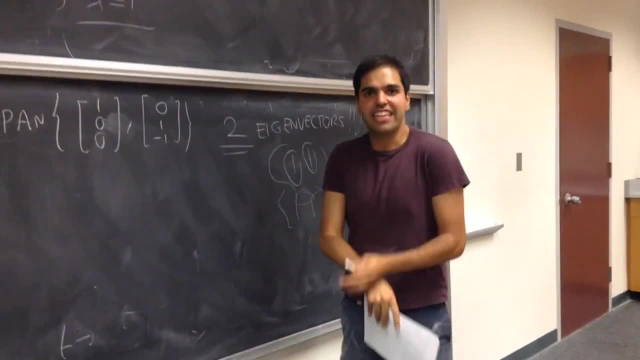 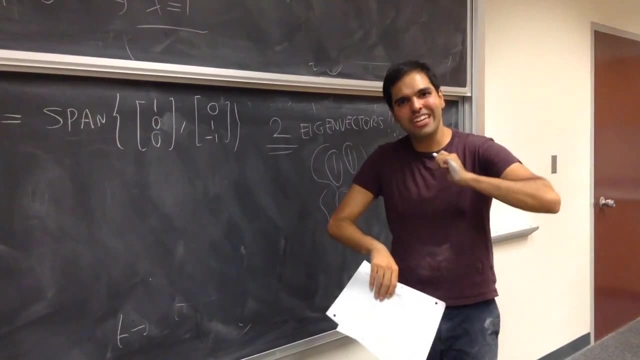 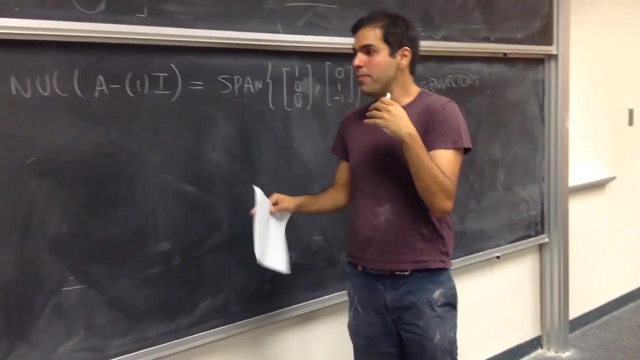 emoji. okay, But wait, what does that tell us? It tells us you cannot put this matrix into a diagonal form. but let's see, we can still put it in a Jordan form, which is slightly better. But now let's maybe analyze this Jordan form a little bit, So suppose you can. 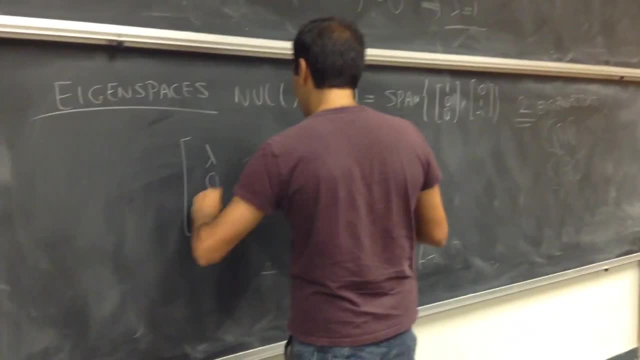 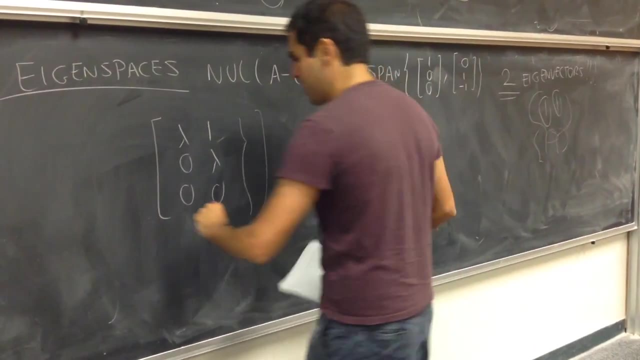 put a matrix in this form. Let's say lambda 0,, 0,, 1,, lambda 0, and whatever some junk here, And suppose the first vector is v1, and the second vector is v2.. By definition of a matrix, 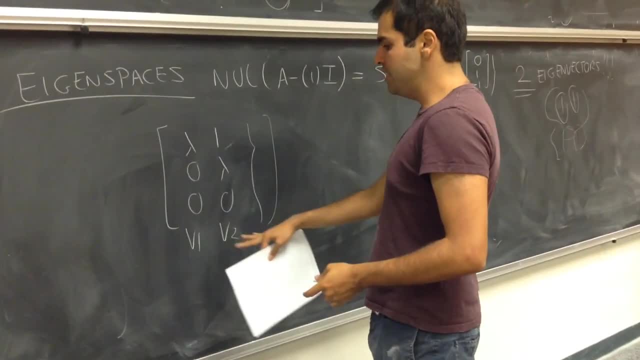 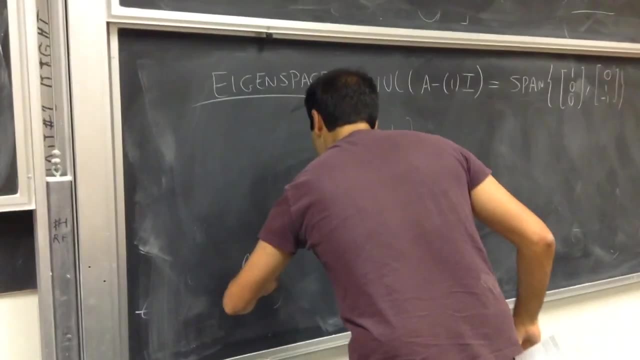 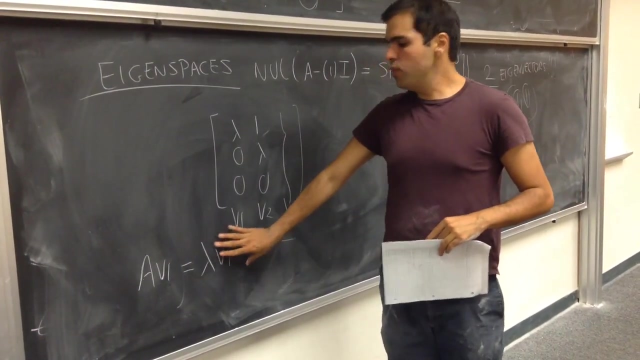 what that tells us is that if you want in the basis v1,, v2, and maybe v3,, we have that a of v1, it's lambda v1. This already tells you that v1 has to be an eigenvector, which means we have to choose. 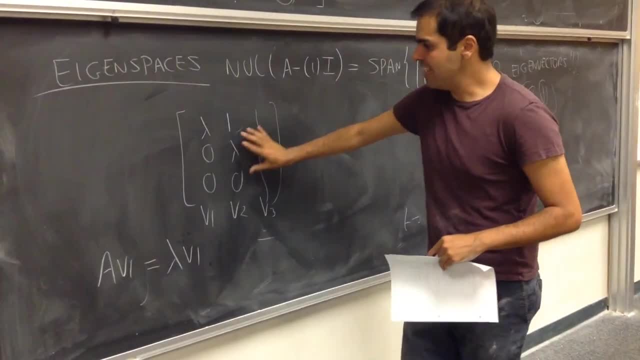 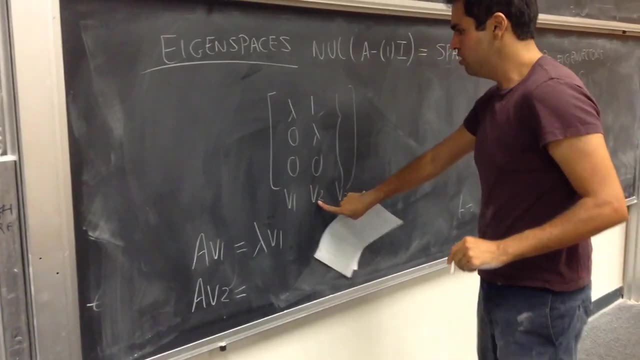 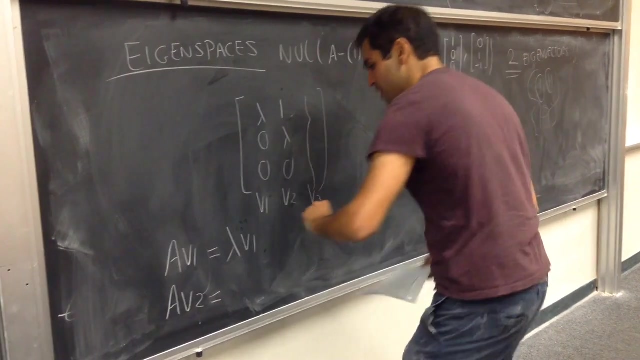 one of those two. okay. On the other hand, let's see what this means. Well, technically this means that if you apply a to v2, so the second column- you get 1 times the first vector plus lambda times the second vector, which is v1 plus lambda times the second vector. 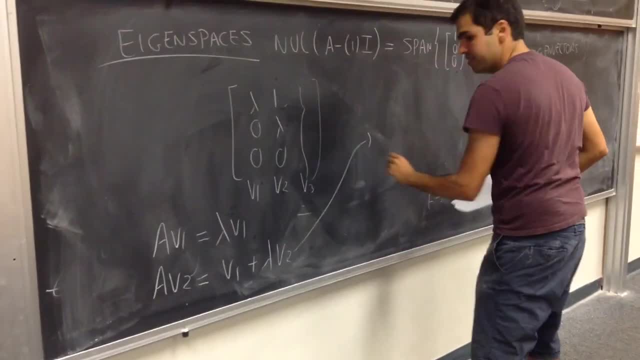 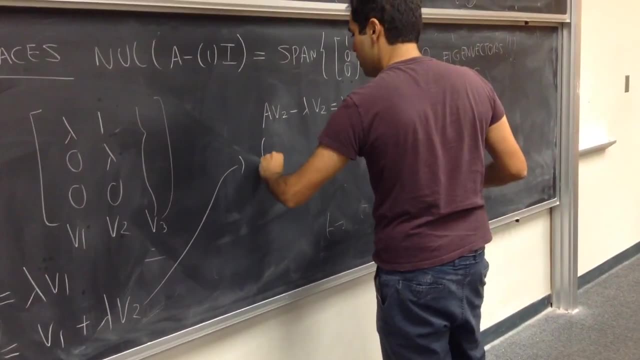 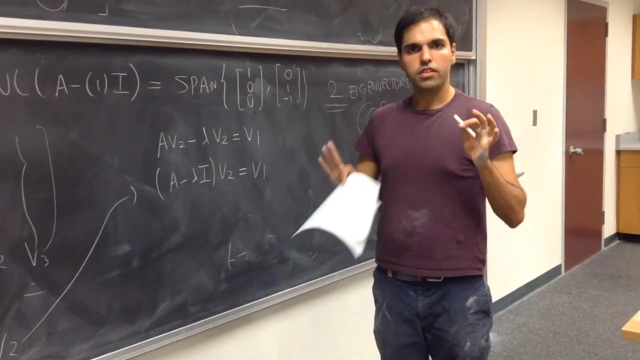 which is lambda v2.. Let's rewrite this: You get ab2 minus lambda v2 equals to v1.. In other words, a minus lambda i v2 equals to v1.. And this is very, very important. First of all, 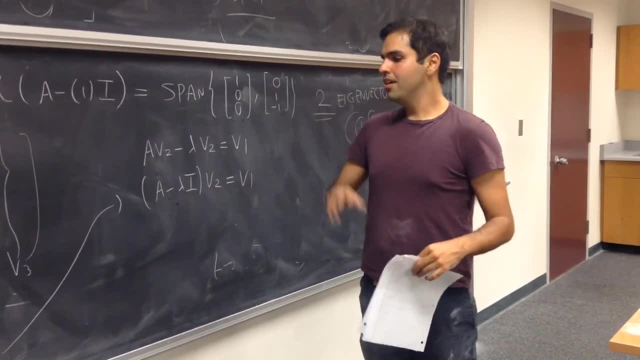 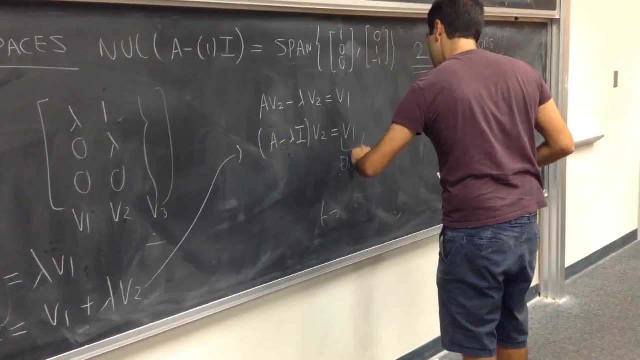 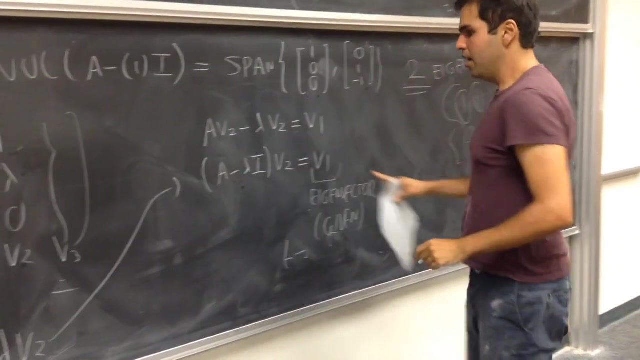 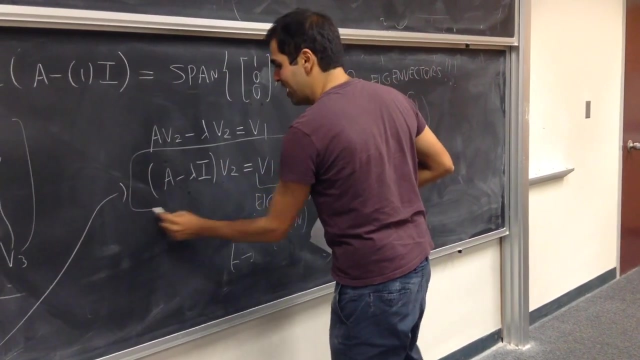 notice this: a minus lambda. i appears again And remember the following: v1 is an eigenvector, Like f is an eigenvector. l is a constituent factor. 1 plus lambda- i Right, It's given. What does that tell us? It tells us that to find v2, you have to solve the following equation: 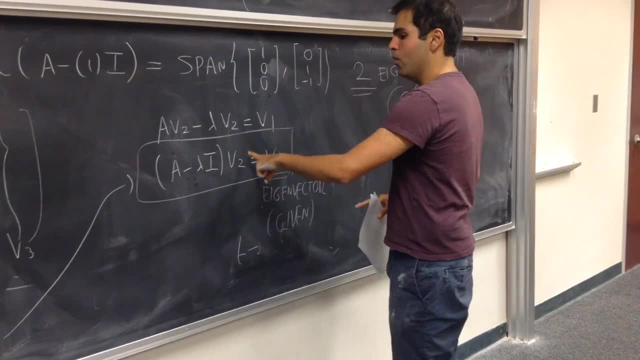 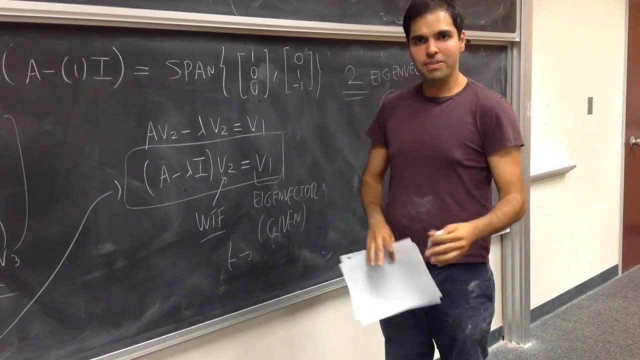 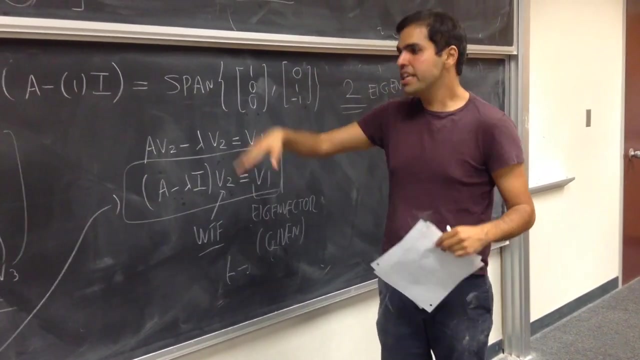 a minus lambda i, that's given, equals to an eigenvector, which means—no, exactly this. It's given, It's given v1 equals a zur트 τους, which is, according to the derivative, an eigenvector. you have to sort of back-solve this equation to get another vector for a. 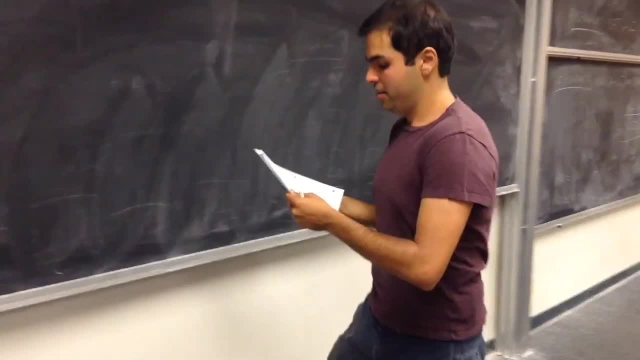 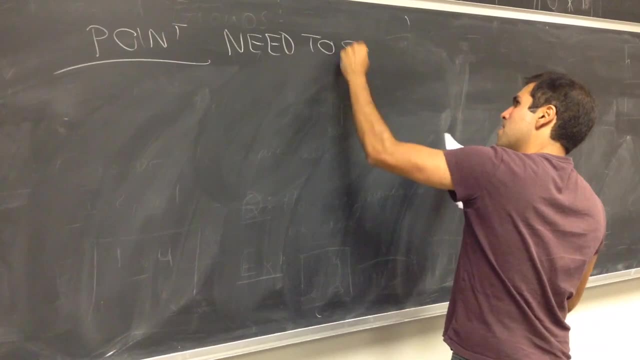 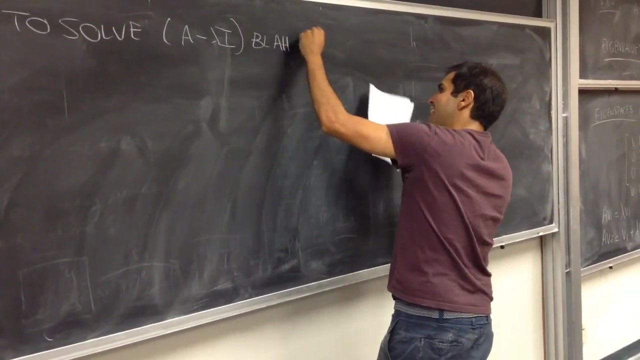 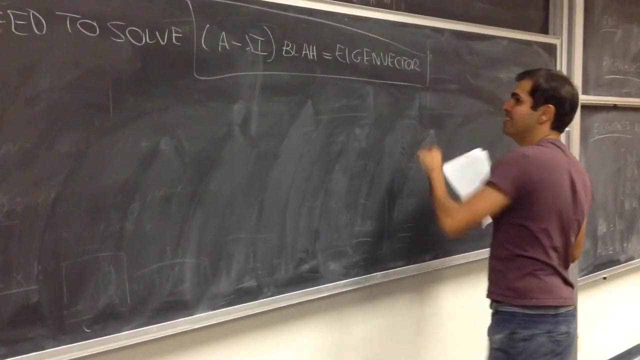 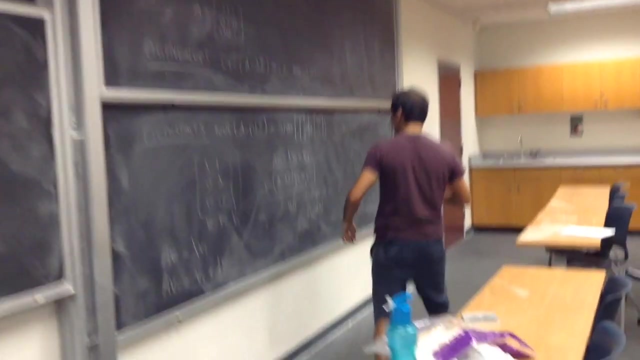 gendron block, And so let's do this. We need to solve: a minus lambda i times blah equals two eigenvectors. This is the magic equation, if you like. Okay, but look, sorry, go back to this equation Here. we really just have two eigenvectors. So basically, let's just 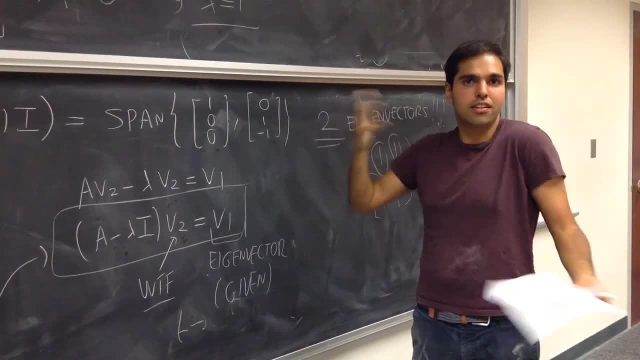 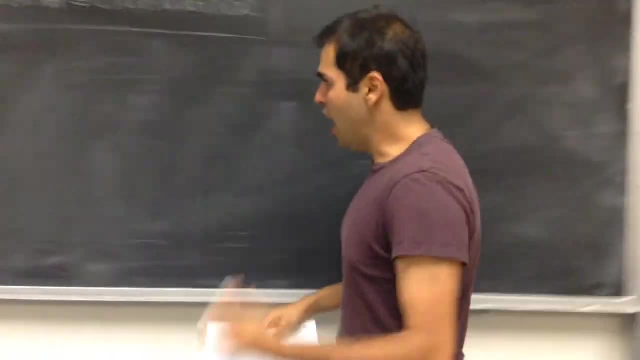 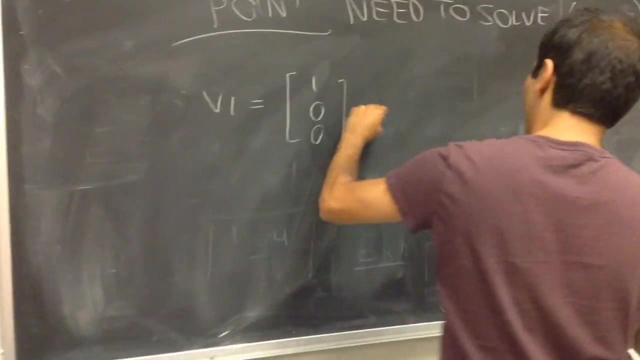 start with one and let's see if we can back-solve it. If we can, great, we found another gendron vector, if you want, Okay. So how about let's start with v1 being 1, 0, 0, and solve. let v1 be 1, 0, 0, and solve. 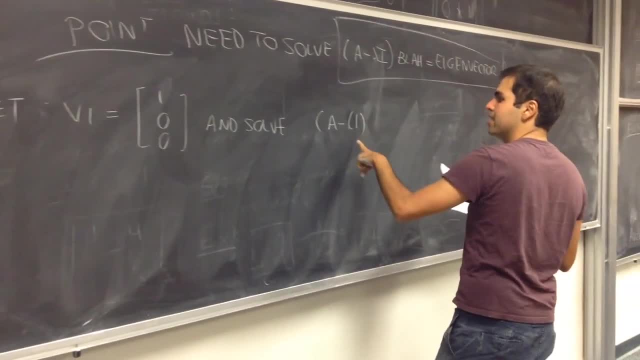 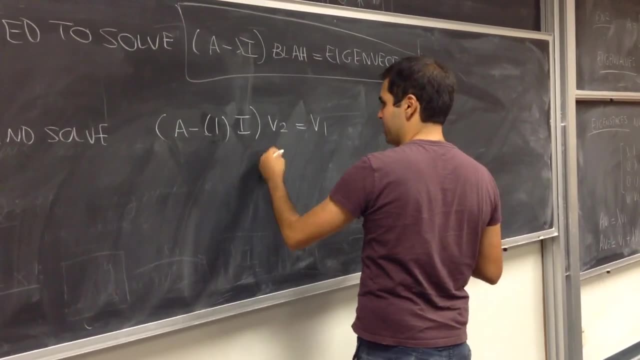 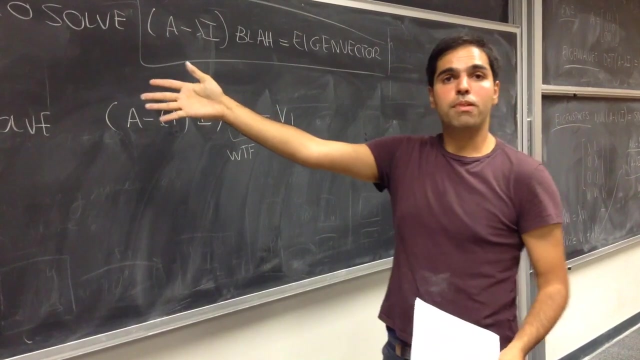 a minus i, so maybe my a minus the eigenvalue, which is 1, i. v2 equals to v1.. Again, remember, we want to find this Okay. And again, by the way, it's completely random why it shows 1,, 0,, 0.. You could have tried. 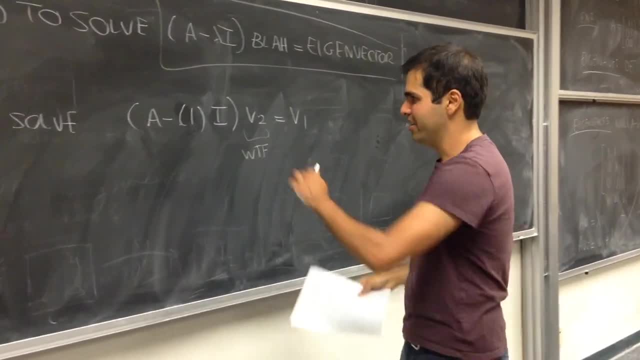 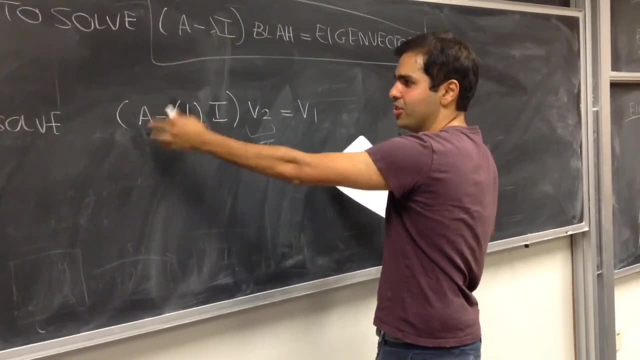 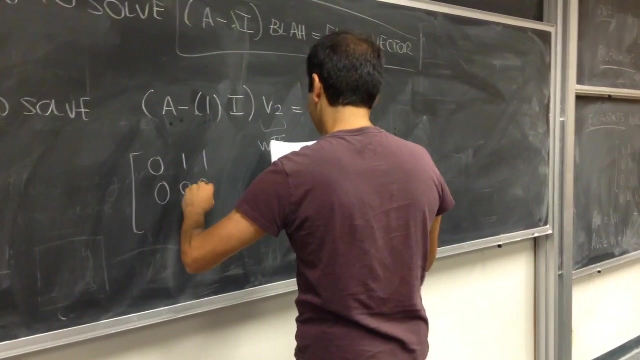 with the other one. but you will see, the other one has no solution. But the nice thing is we've already, you know, in the process of finding the eigenvectors you already found a minus. i So suppose you do this and you get 0, 1, 1, 0, 0, 0, 0, 0, 0, v2 equals to: 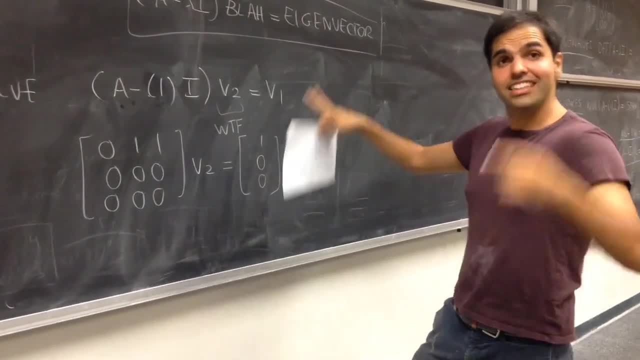 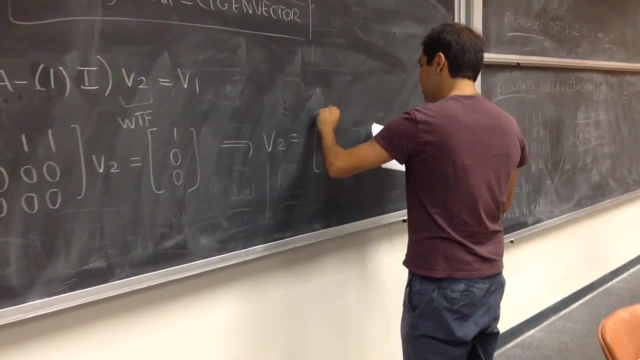 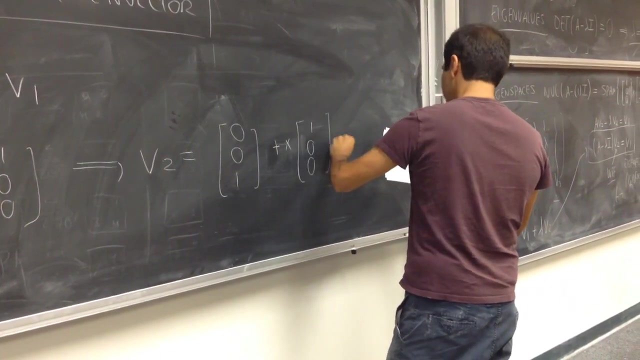 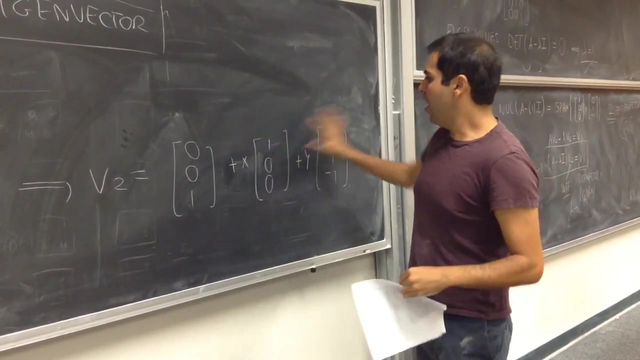 1, 0, 0.. If you do that, you indeed get a solution, Namely, if you gaussian eliminate, you get v2 is 0, 0, 1, plus x, 1, 0, 0, plus y, 0, 1, minus 1.. And it turns out all this is just. 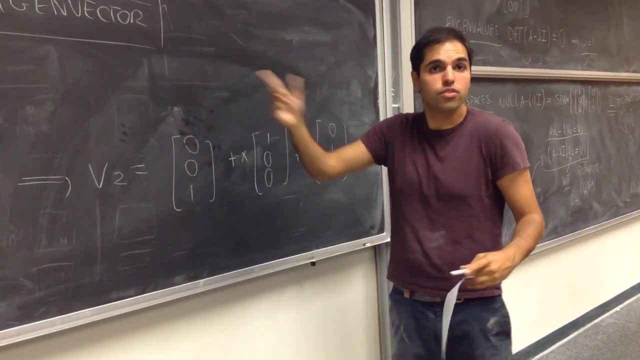 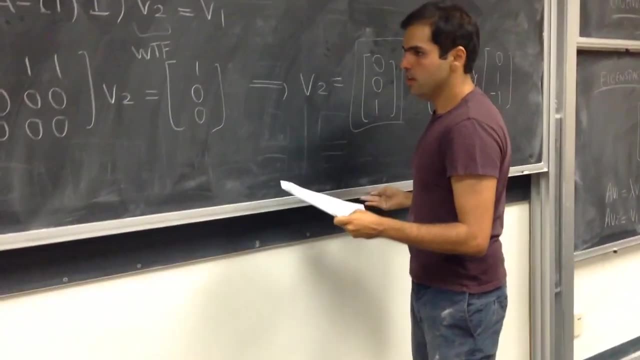 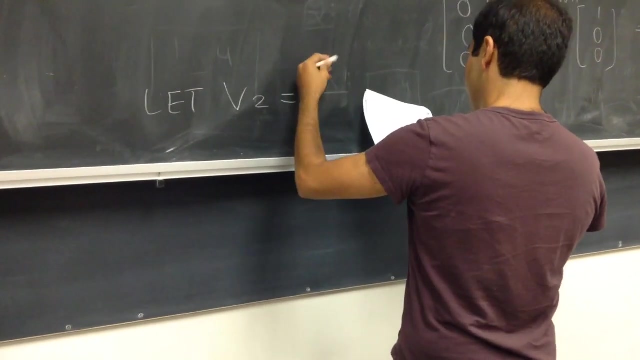 garbage. You just need one of them because you just need one vector. You just need one vector. So how about we just choose the easiest one: 0, 0, 1.. So again, let v2 be 0, 0, 1.. And again, that's great, because it tells us that a has the 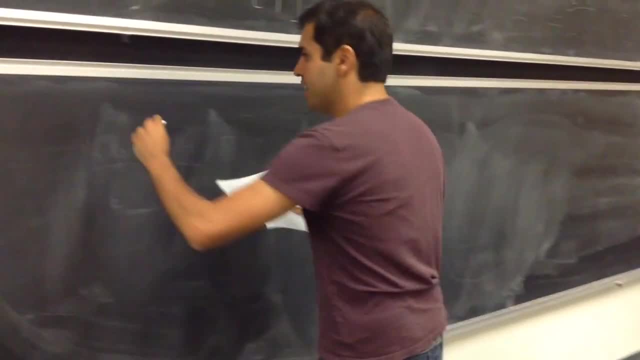 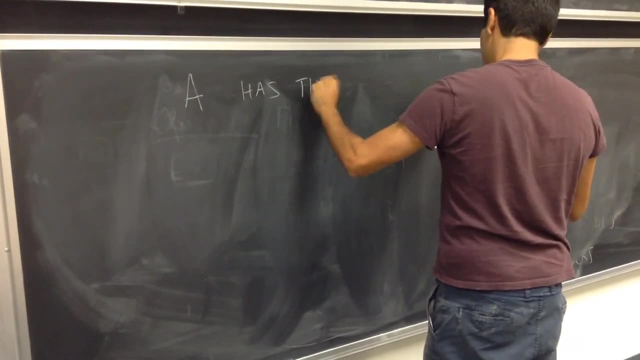 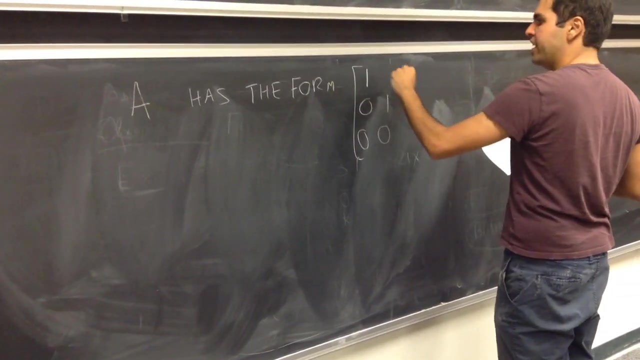 following form. So it tells us already that a, you know, has the form. So it can be put in the form Again: eigenvalue 1, 1, 0, 0, 0, and the above thing is 1.. Sorry for using 1,, but if the 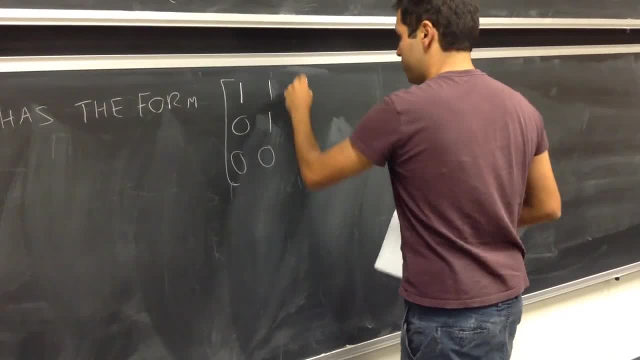 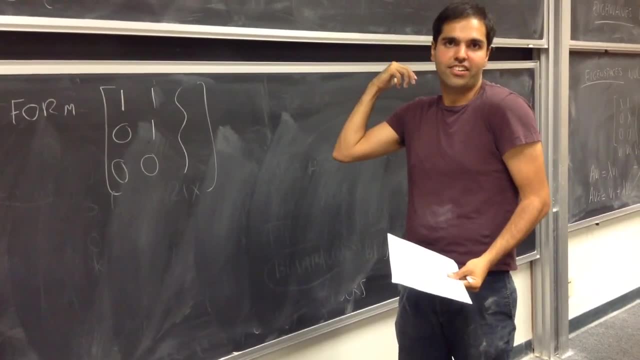 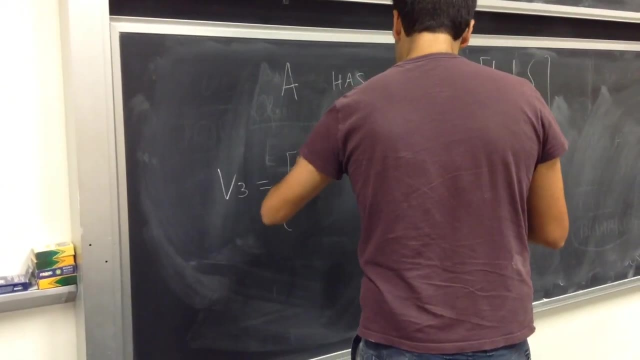 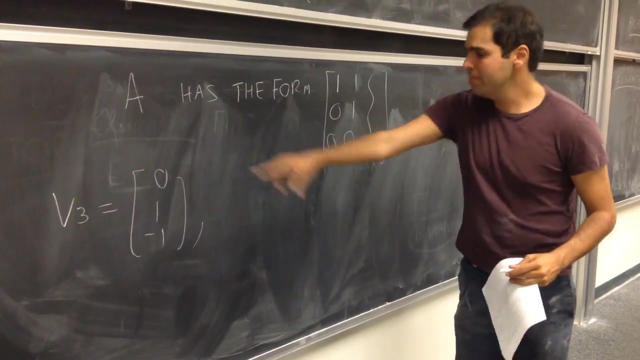 eigenvalue were 2,. it was 2,, 2,, 1, and some other junk. But look, for the rest, we can just use the other eigenvector. So let v3 be the other eigenvector: 0,, 0,, 1, minus 1.. And then what this really tells us is that the last term can be put. 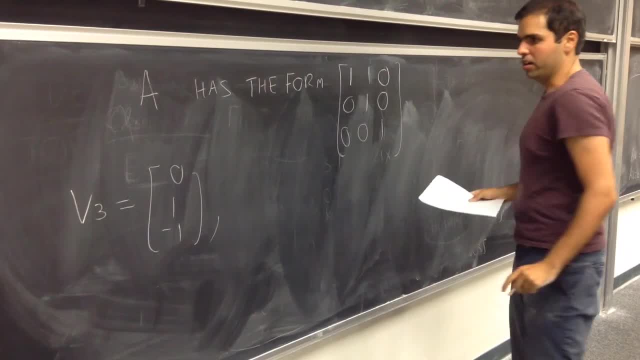 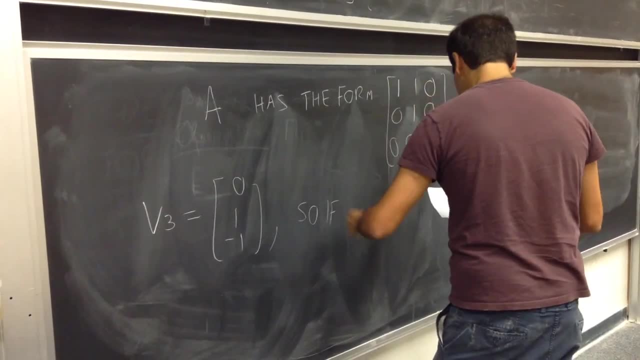 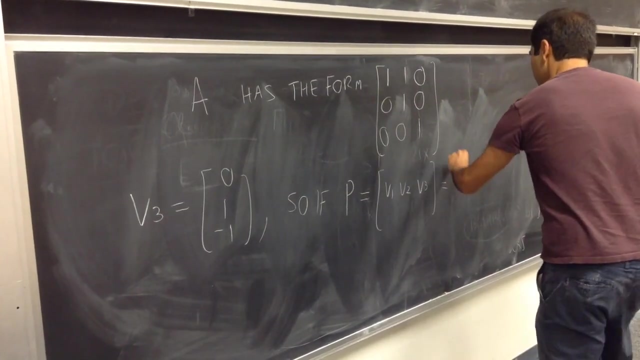 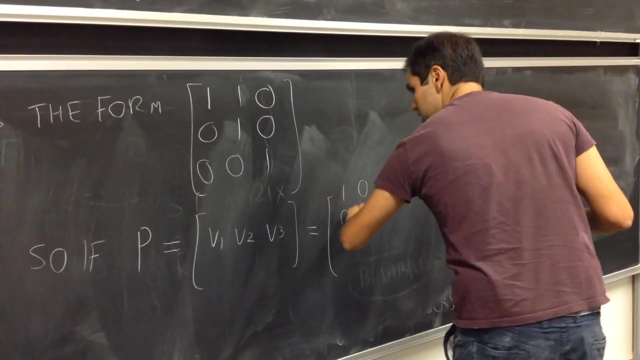 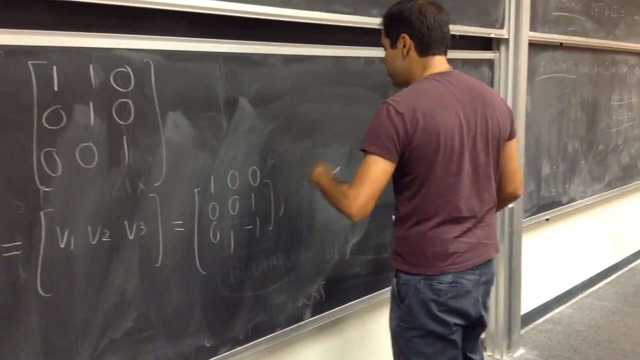 in the just diagonal form, 0, 0, 1.. In other words, so if p, if you let p, equals to v1, v2, v3, which is 1, 0, 0.. v2, 0, 0, 1, and 0, 1, minus 1.. Then before we had a equals to pdp inverse. but now, since 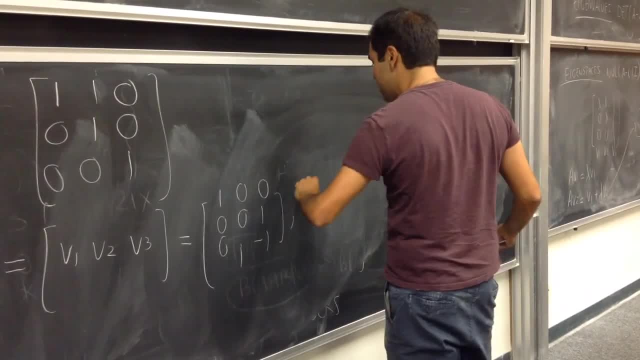 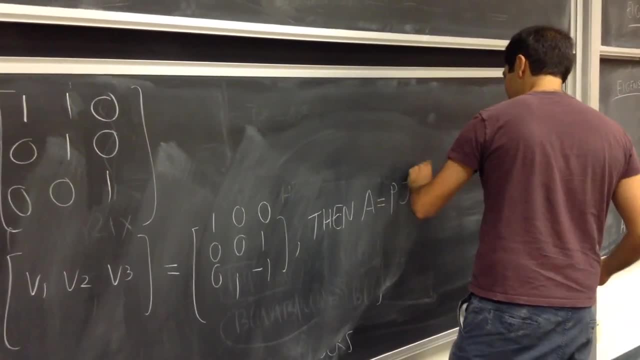 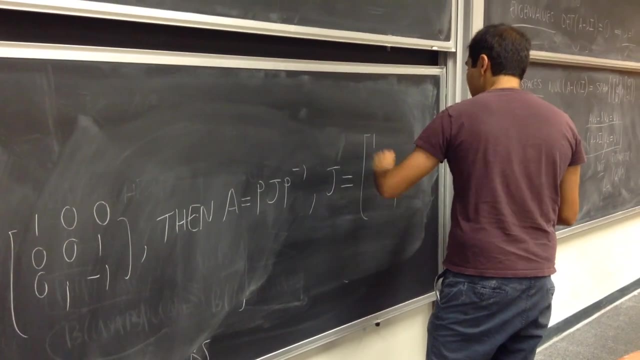 we're talking about Jordan, you know. we want to say a equals to pjp inverse, That's right, like peanut butter and jelly And j equals to, again the matrix. So 1,, 1,, 1, except there's this additional 1 here. 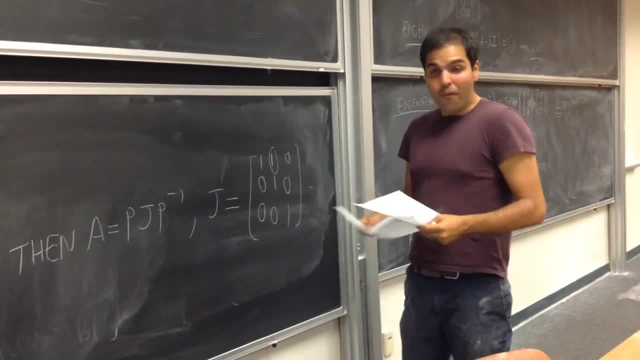 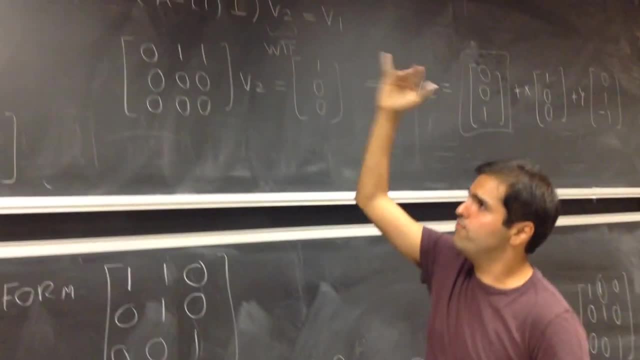 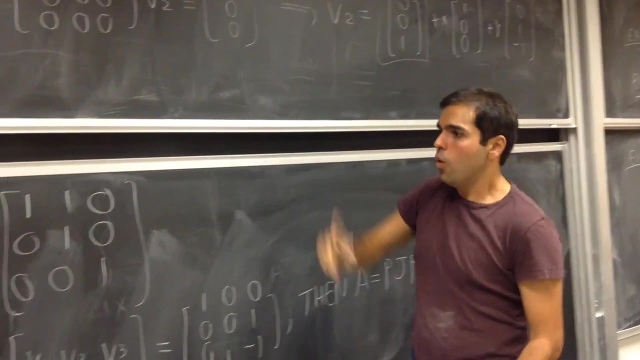 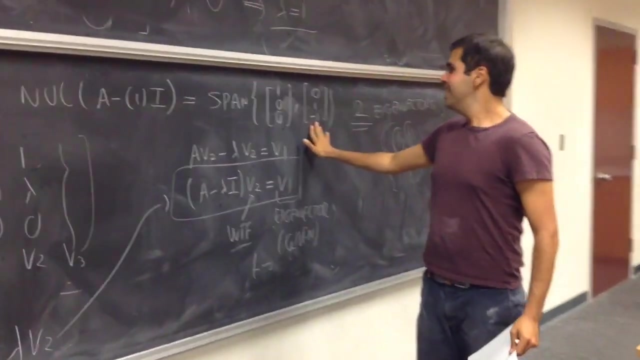 Wonderful. OK, Just one more comment, because so here we solved. we've picked one eigenvector and we solved a minus i. v2 equals to v1.. What if we picked the other eigenvector here, 0, 1, minus 1.. What would happen? 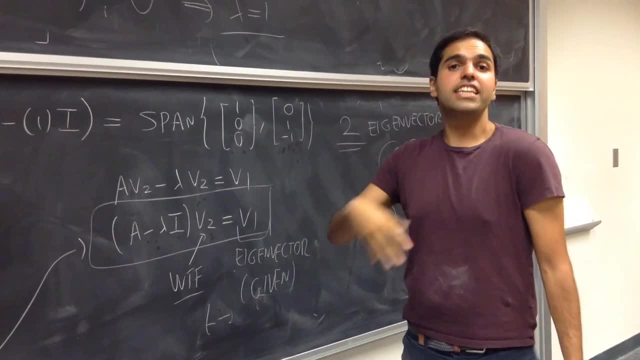 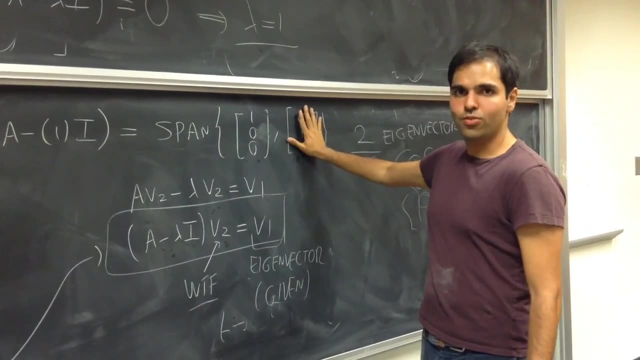 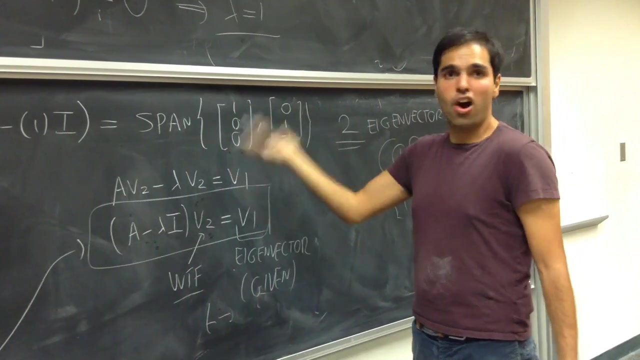 What would happen if we did this procedure? We would find that the equation has no solution, which tells us that since the equation has no solution, this vector doesn't work. So really, the general procedure is find the eigenvectors and just back, solve as much as. 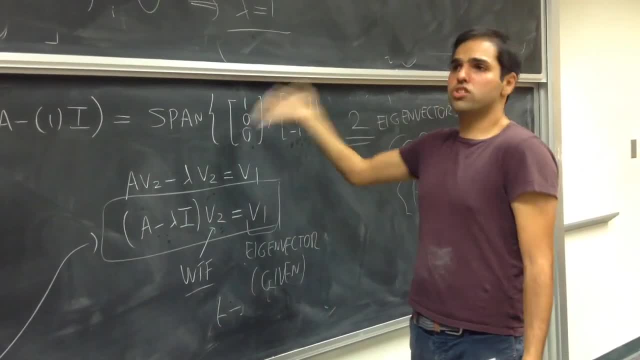 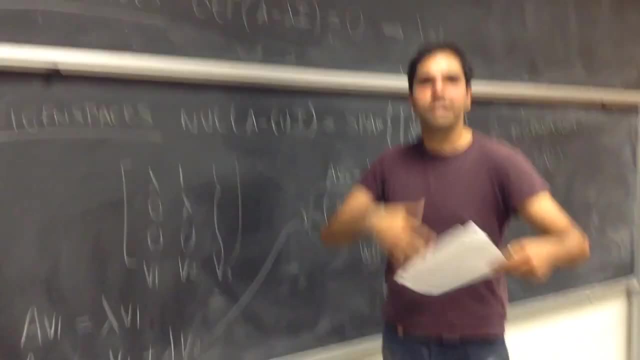 you can, If one vector doesn't work, just try out the other vector. That's why I'm saying this method isn't quite rigorous, because it turns out there's this theory which tells exactly what vector to pick. but, to be honest, that just went over my head. 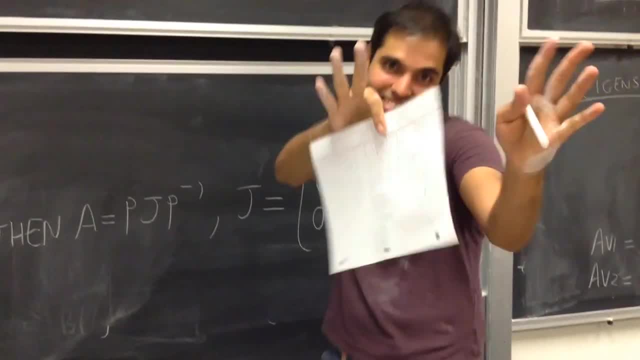 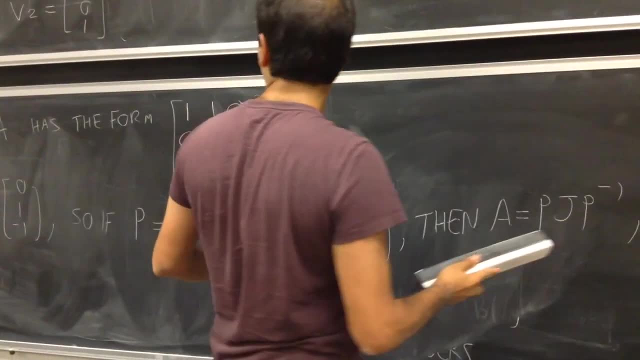 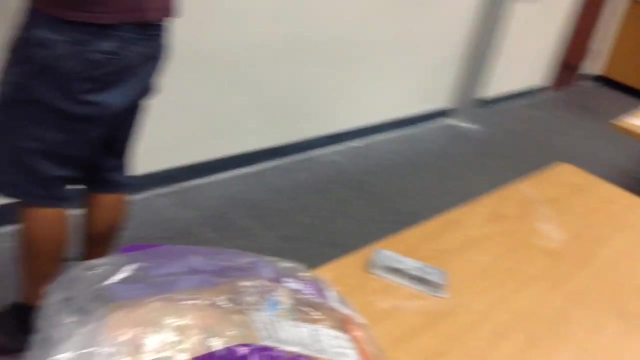 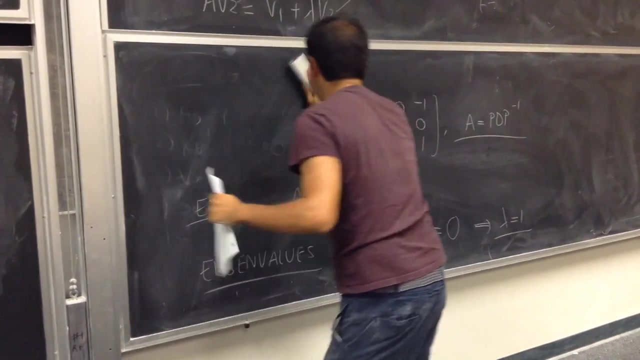 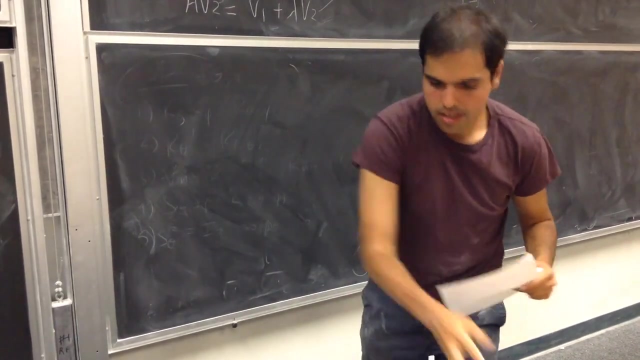 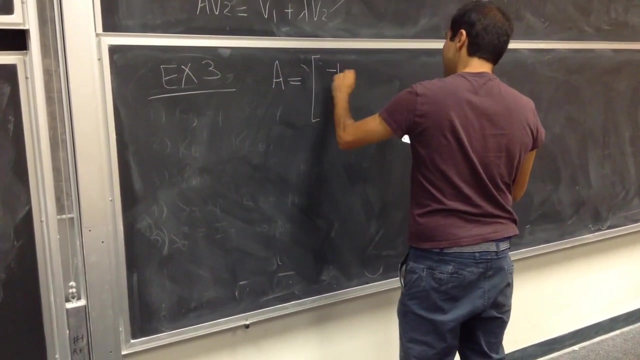 Last but not least, we're not quite done. sorry, but what about the other case, the more general case? Well, let me see. which platform can I use This one? What about the worst case scenario, Example 3.. What if your a equals to minus 1, minus 1, 0, minus 1, 0, 0, minus 1, minus 2, 0?? 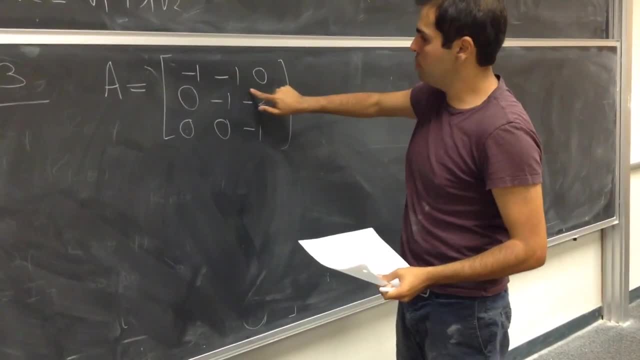 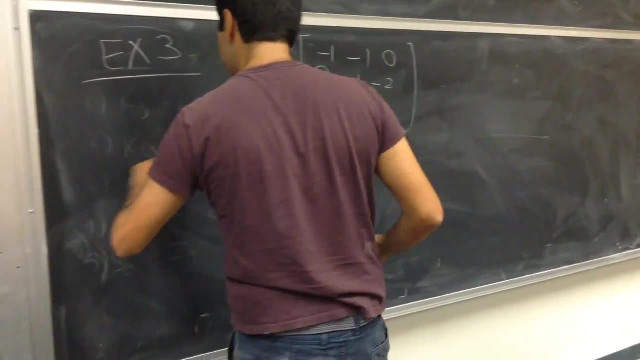 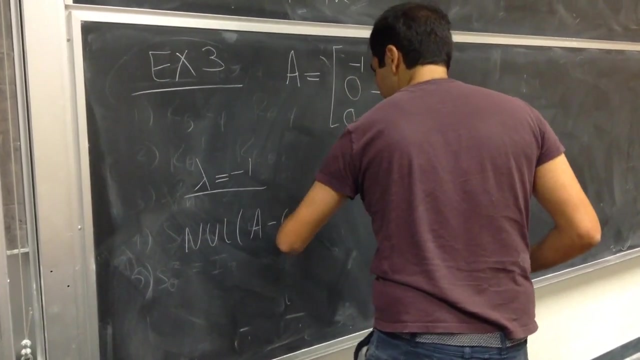 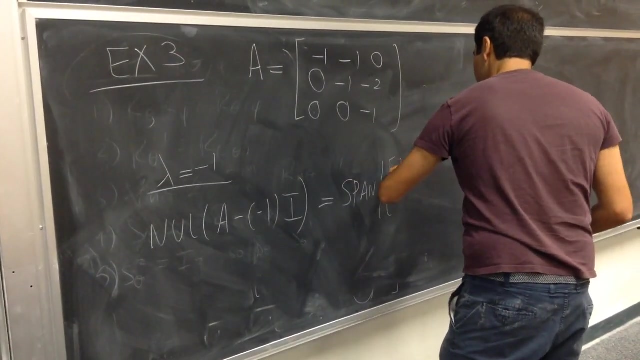 Again, not the Jordan block, because those numbers need to be 1.. It doesn't count as Jordan block. So let's see you do the eigenvalues, then you find lambda equals to minus 1, and for the eigenvectors no space of A minus lambda. I let's say you have the span of 1, 0, 0,. 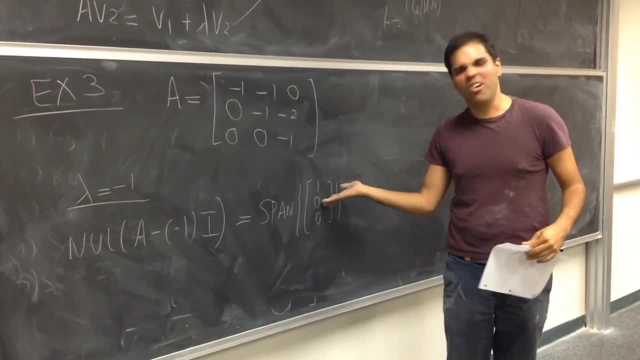 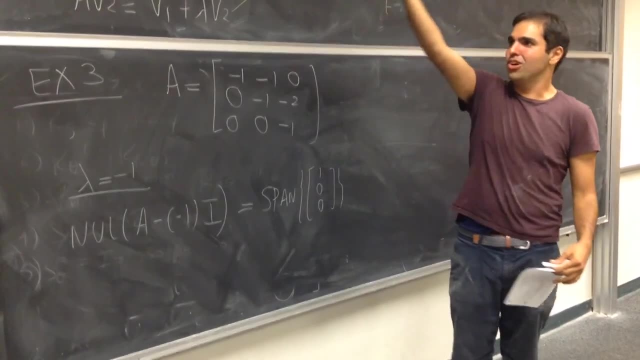 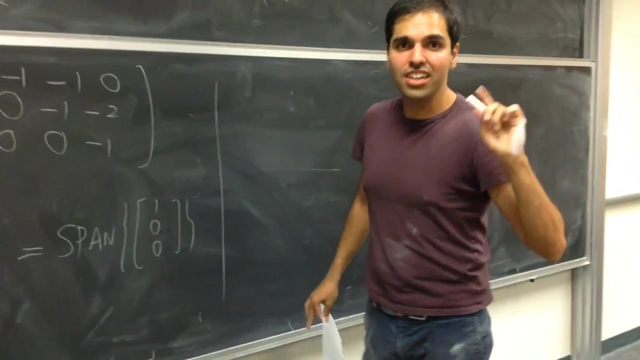 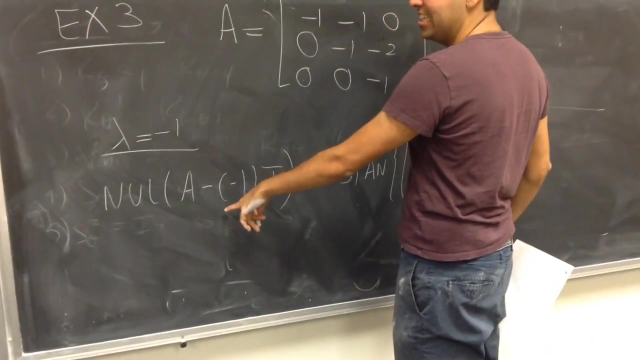 this is horrible Because you only have one eigenvector, so for sure it's not diagonalizable and also we couldn't use the technique before It turns out. even with one eigenvector, you can still put it in Jordan form: Yay, And, by the way, some people like to use lambda: I minus A. 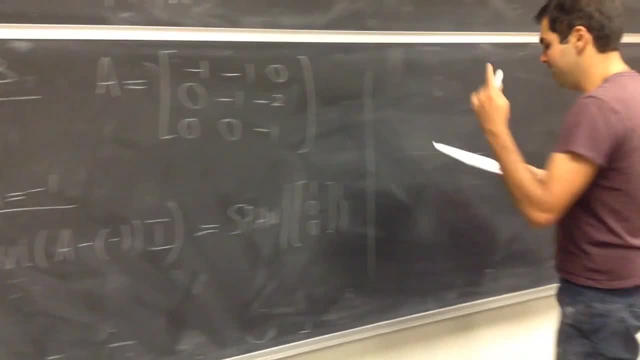 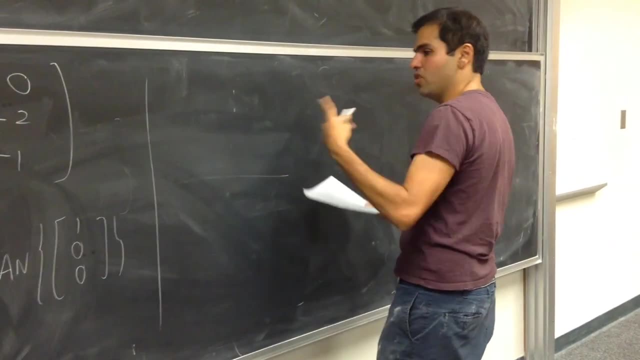 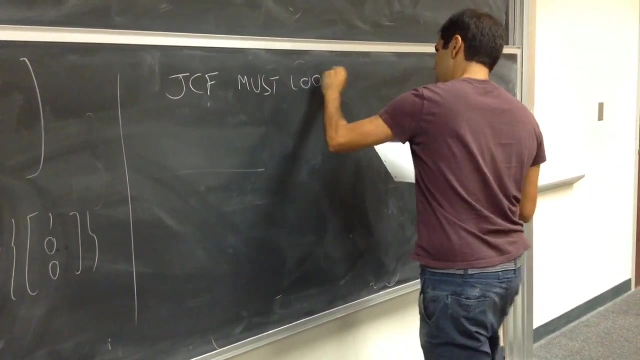 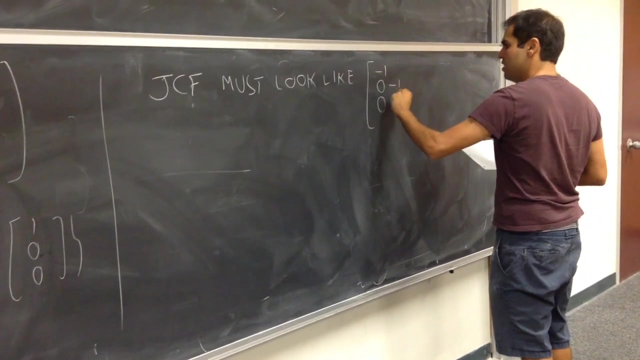 this technique only works with A minus lambda I, otherwise it's just messed up. What does it tell us? It tells us really already that the Jordan canonical form must look like this: Minus 1, 0, 0, and then minus 1, 0, and we have just one repeated eigenvector and everything. 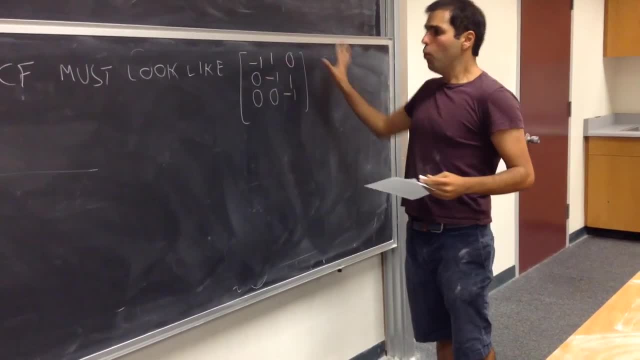 above already has to be 1.. What does that mean in terms of what we are trying to solve technically? if we lay the equation out, basically whatever the vector gets to, we don't get the result. So we can't. 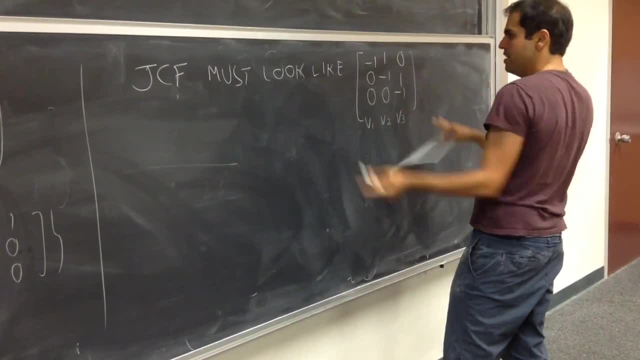 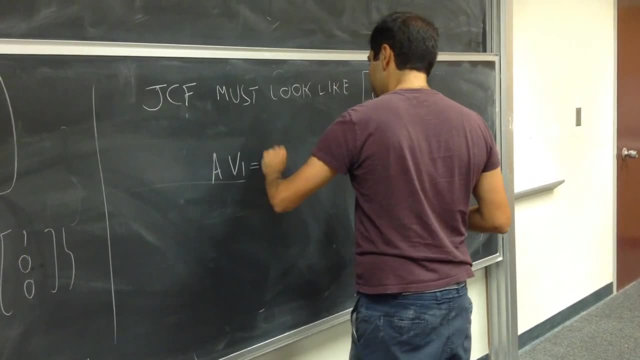 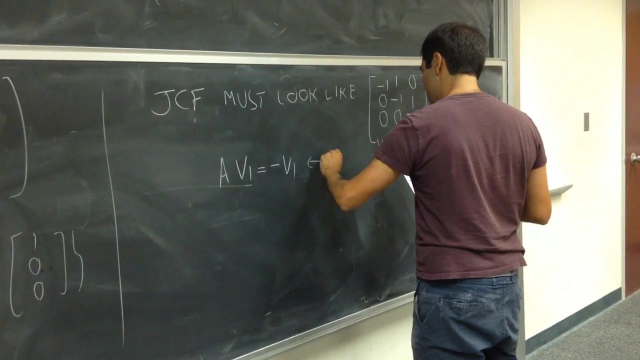 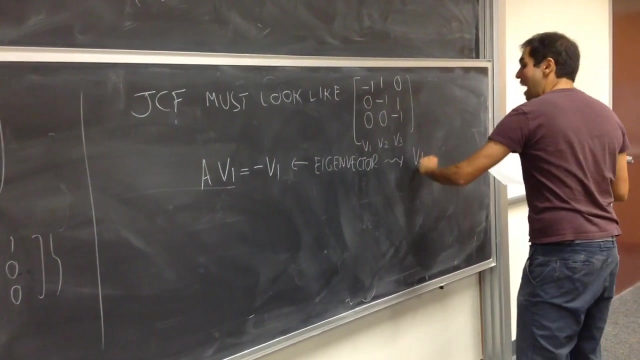 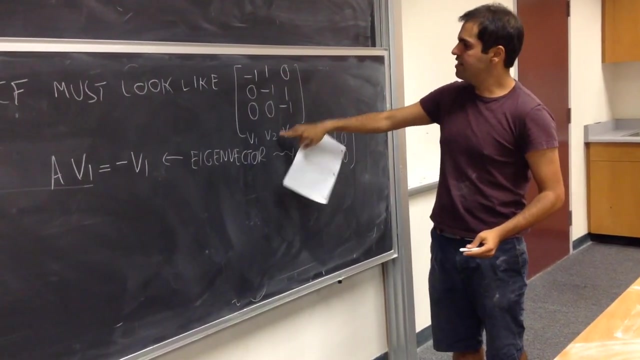 let v1,, v2, and v3 be the three vectors. it tells us already that av1 equals to minus v1, which already tells us that v1 has to be an eigenvector, which means that you have to pick v1 to be. All right, let's continue. What does that mean? It means that 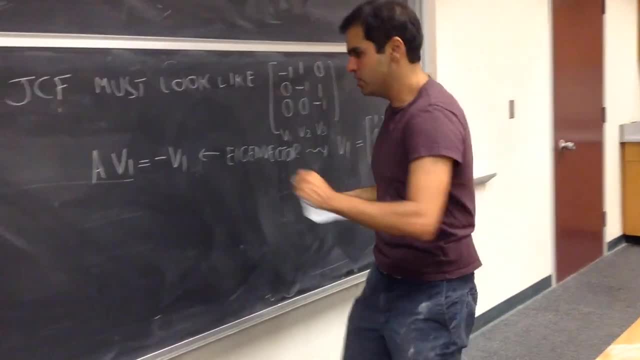 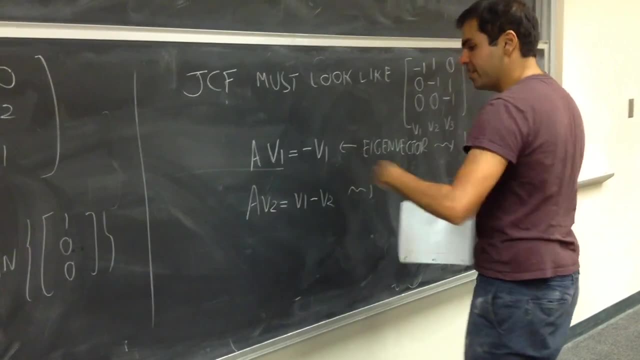 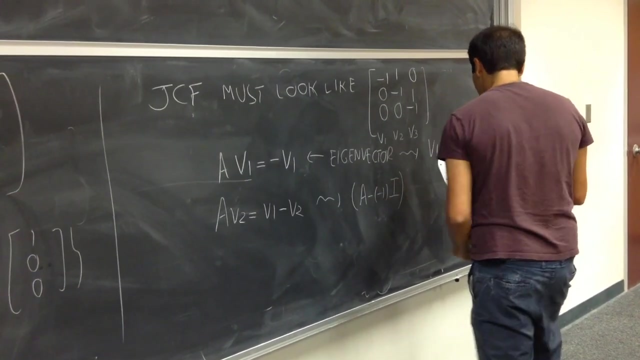 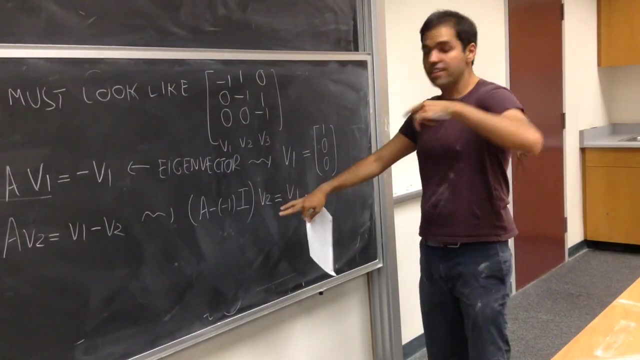 av2 equals to v1 minus v2.. And, just as before, you can reorder this equation and you find a minus minus 1i. v2 equals to v1.. v1.. But that's great because it's basically the same procedure as before. 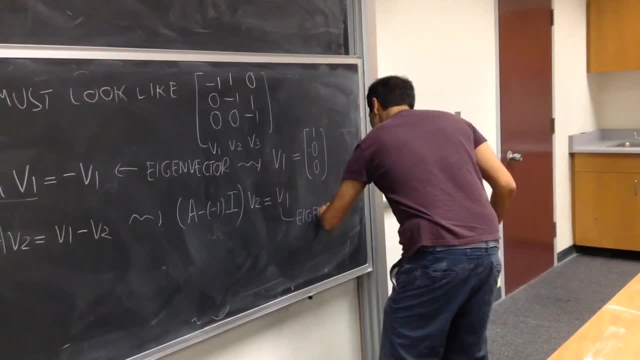 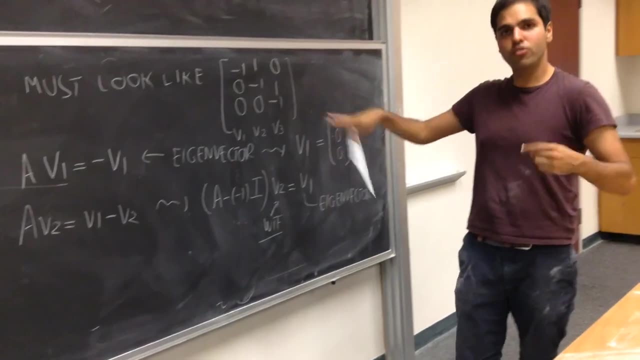 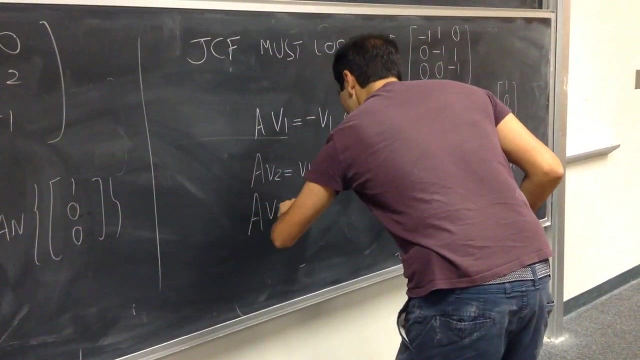 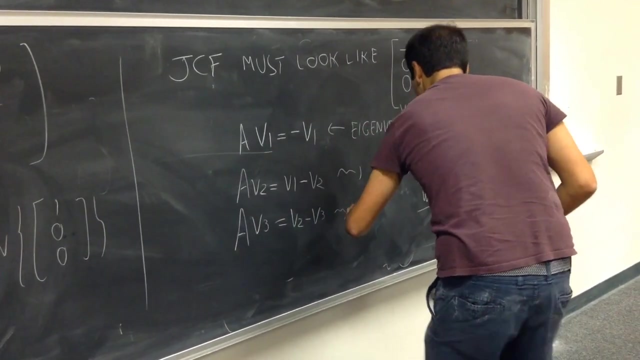 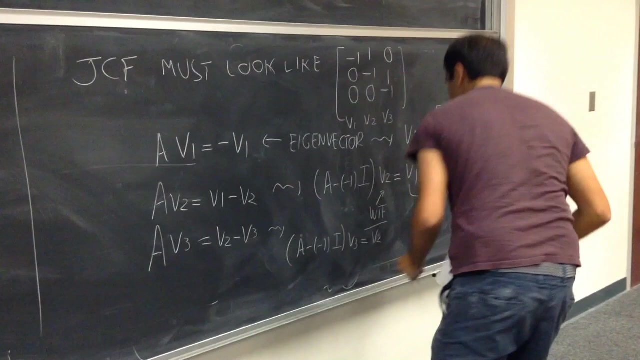 because this is an eigenvector and this we want to find Again. so you have to back solve again. What about the last part? It's actually pretty similar. av3 will become v2-v3, which again tells you that a-1i v3 equals to v2.. But look you already. 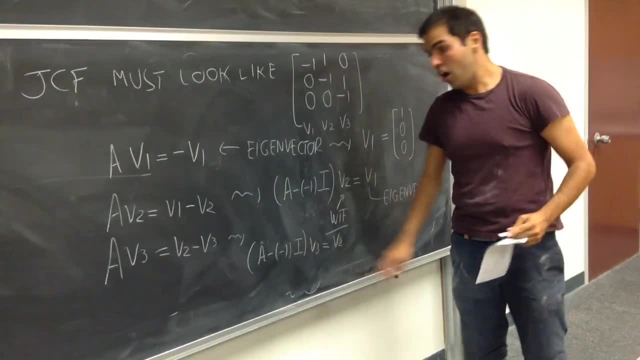 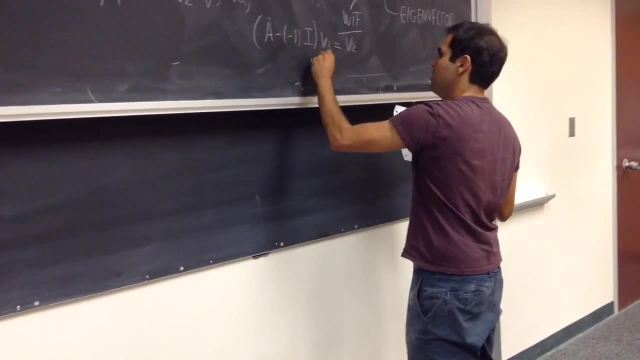 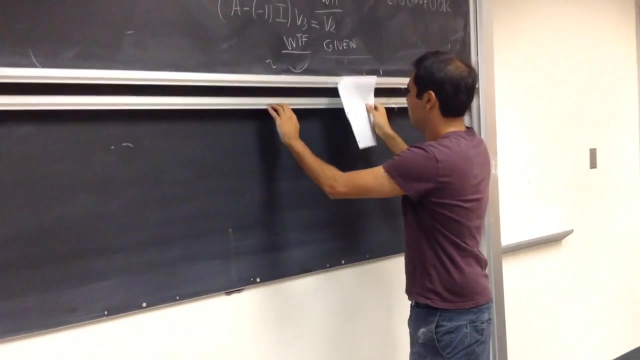 know v2 from this equation, which means all you need to do is again back solve this equation to find v3.. Again, this is one to find and this is given. So you see, you have to back solve a lot of stuff And in fact let's do that. Okay, so let's do this procedure. 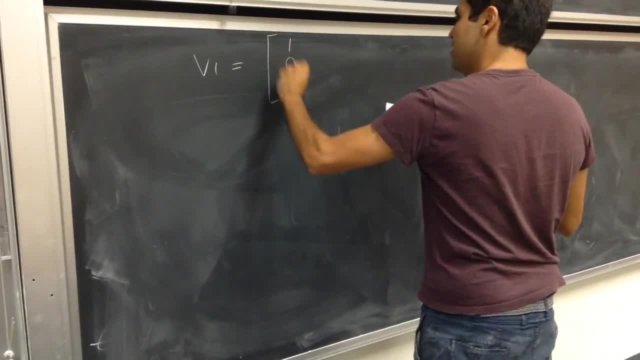 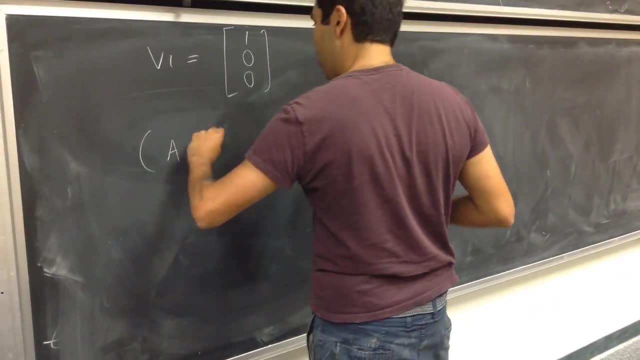 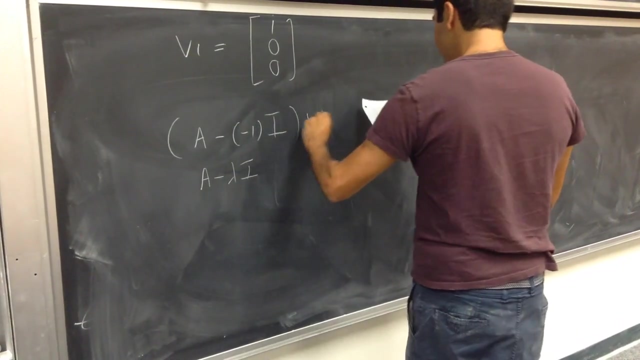 So, as I said, v1 is the eigenvector. the eigenvector, you know, 1, 0, 0. And then, to get the other one, solve a-lambda i. It's always a-lambda i. v2 equals to this junk: 1, 0, 0. And then 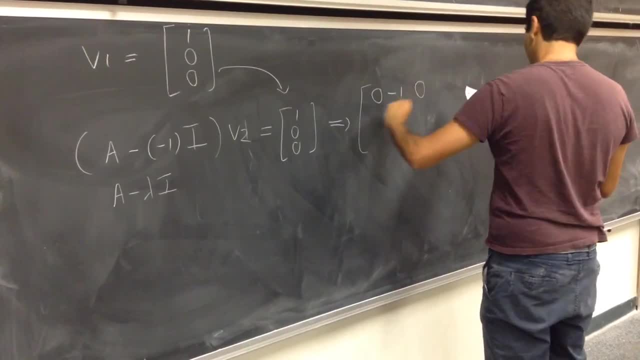 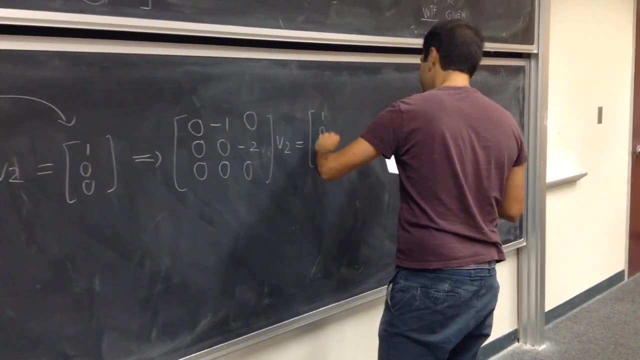 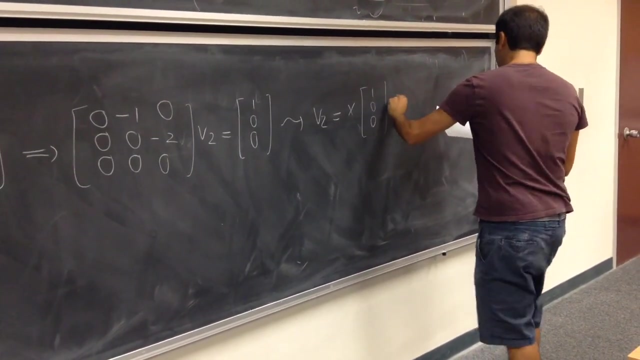 you get 1, 0, 0, which tells you 0 minus 1, 0, 0, 0 minus 2, 0, 0, 0.. v2 equals to 1, 0, 0. You solve that stuff and you get x times 1, 0, 0 plus 0 minus 1, 0. Again, forget that. 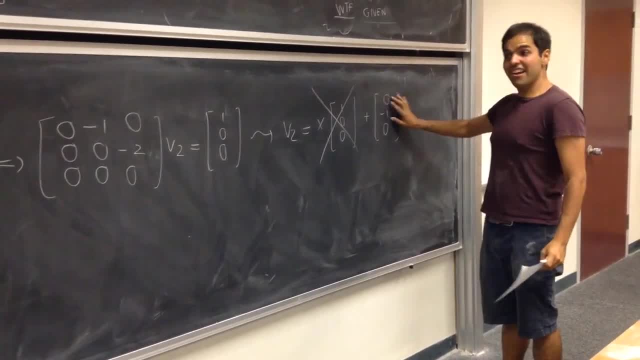 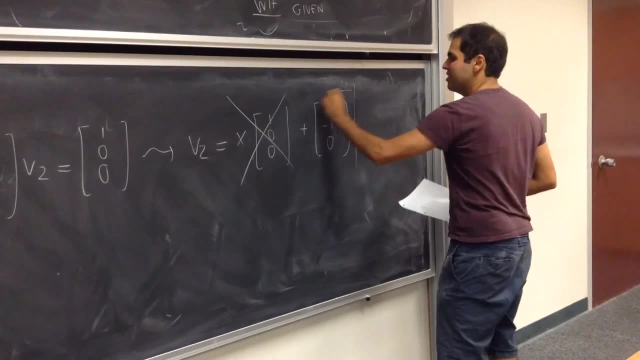 because we want a particular solution. And, very important: do not scale this, Do not write 0, 1, 0.. Because it'll just ruin your thing, It'll ruin your night. So this is our v2.. Great. 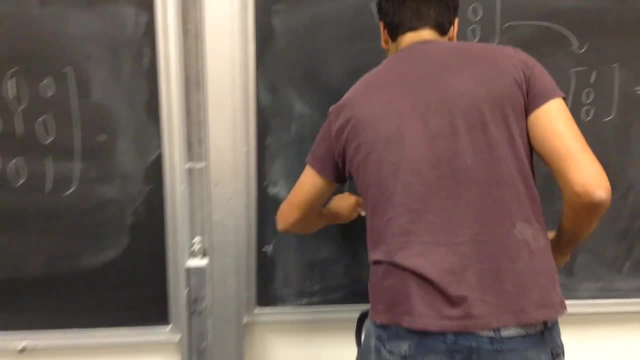 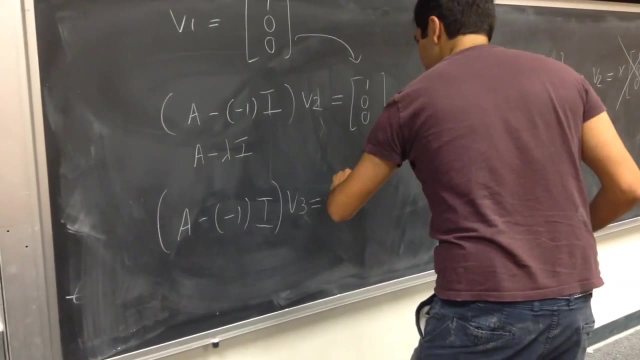 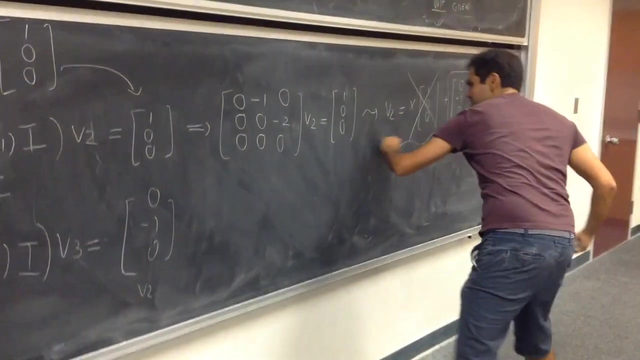 Now that we have v2, let's solve for v3.. a minus minus 1i v3 equals to this v2.. So 0 minus 1, 0.. Again, I want to emphasize: you just put this vector here And again it means: 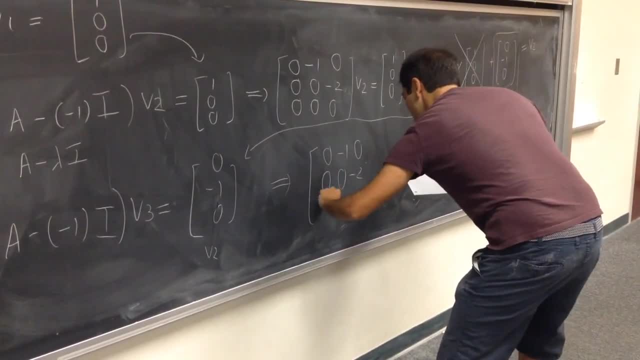 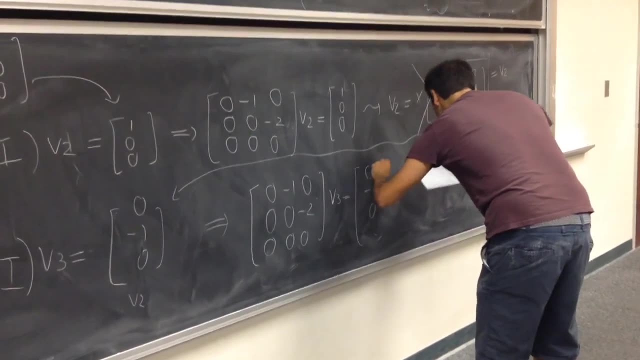 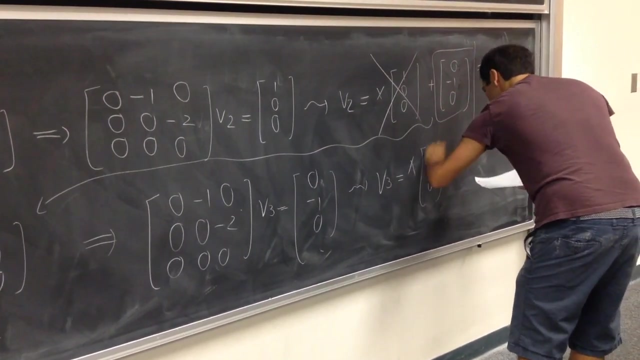 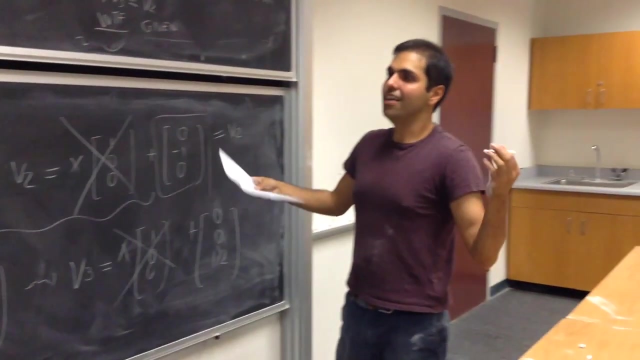 0 minus 1, 0.. 0, 0 minus 2.. 0, 0, 0.. v3 equals to 0 minus 1, 0.. It tells you that v3 is x times 1, 0, 0. You get that plus 0, 0, 1, 1.. This is fantastic because it tells you we're 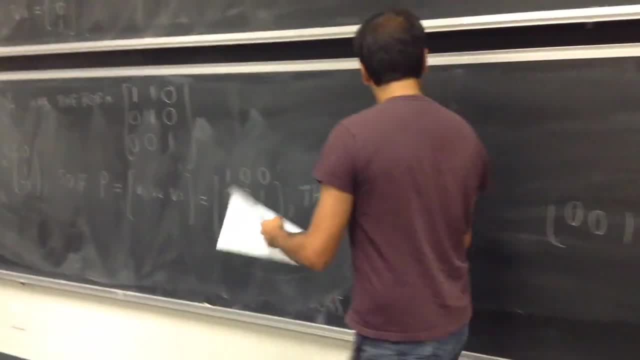 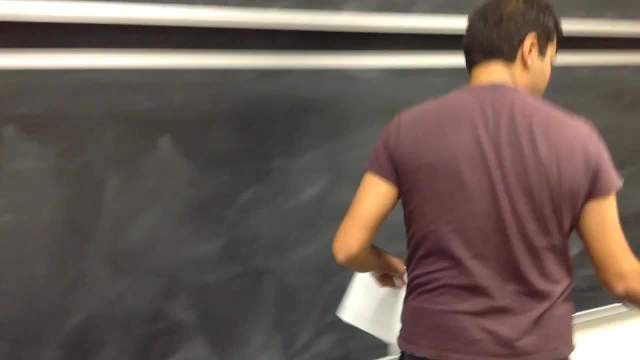 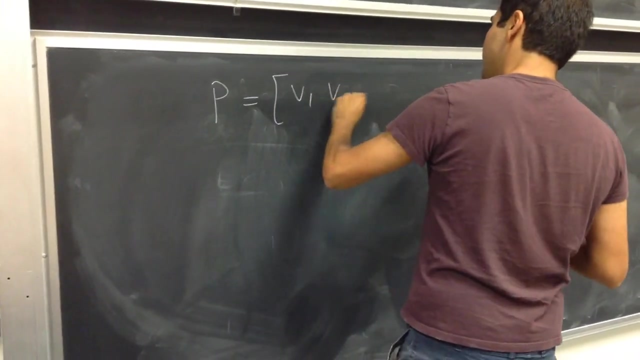 basically done. So you can do that if you define p to be the matrix of all the vectors that we found. So p is the matrix v1, v2, v3.. And important, the order does matter right now, So it's 0,.